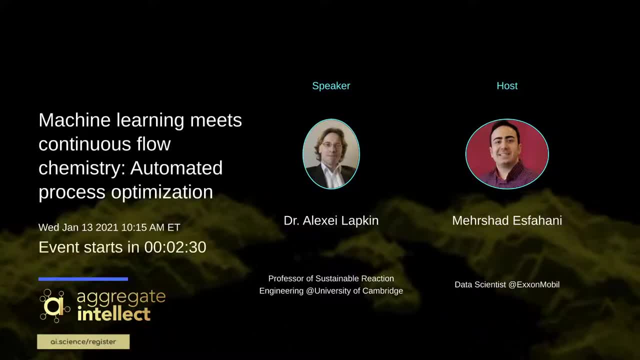 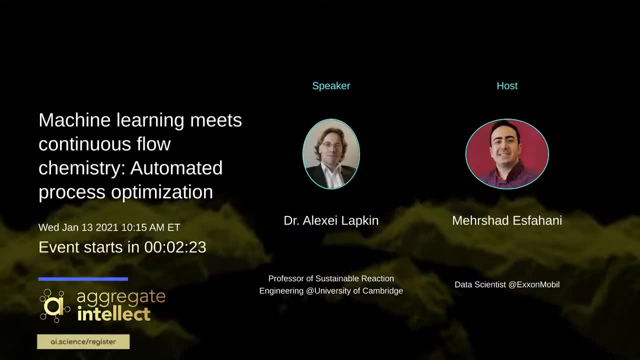 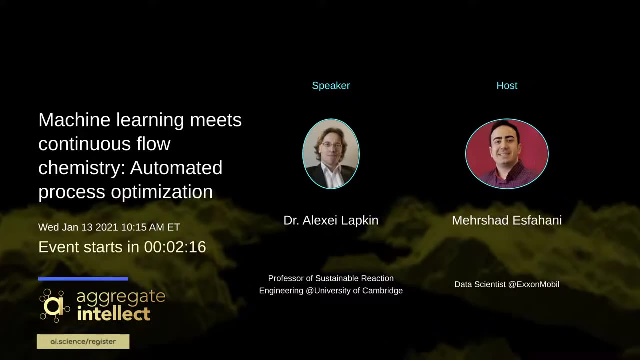 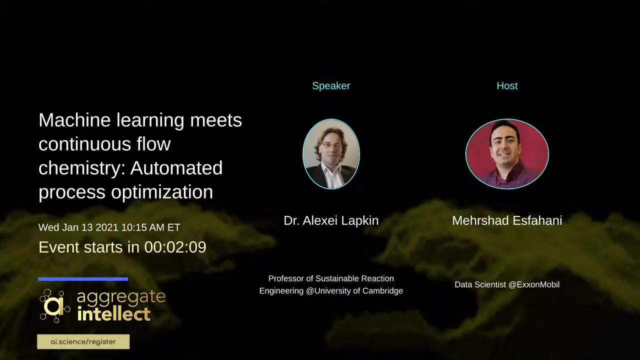 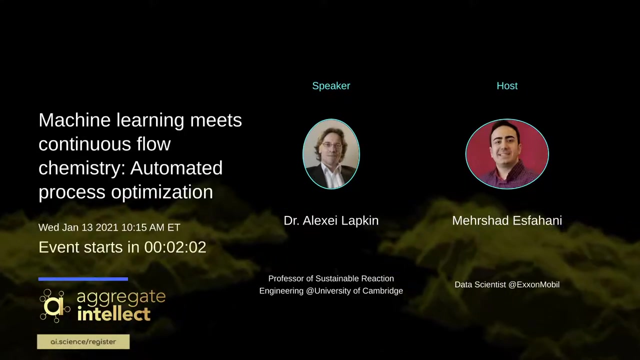 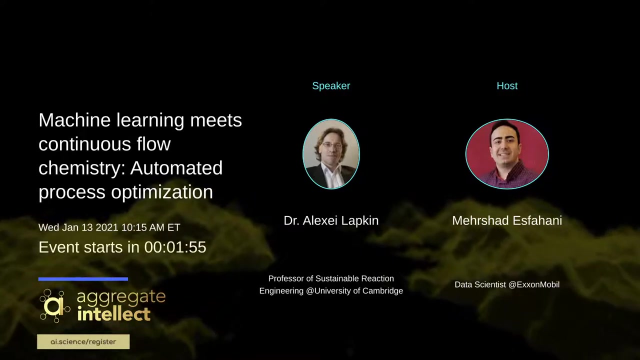 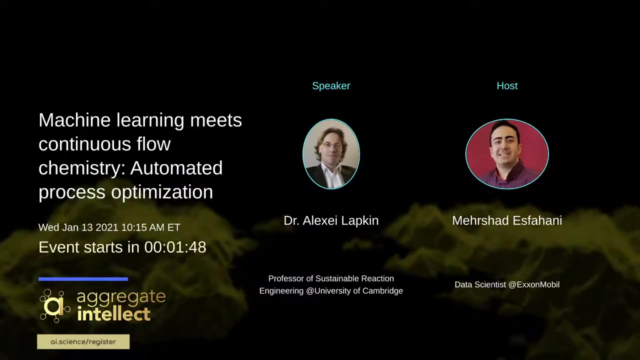 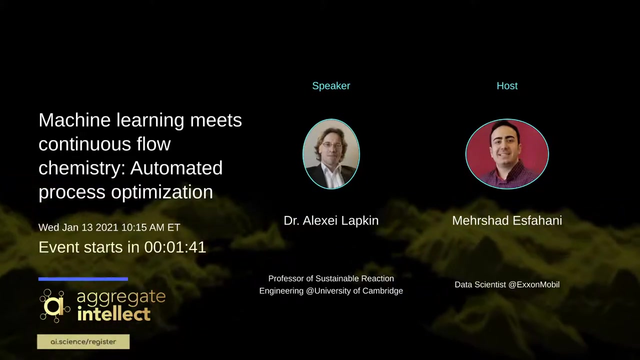 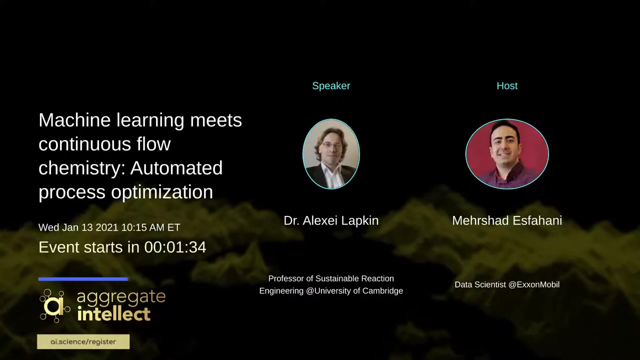 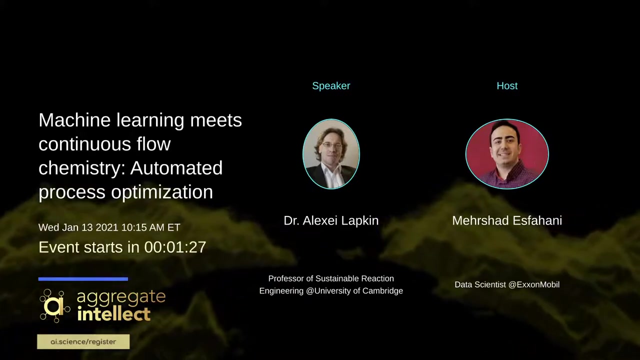 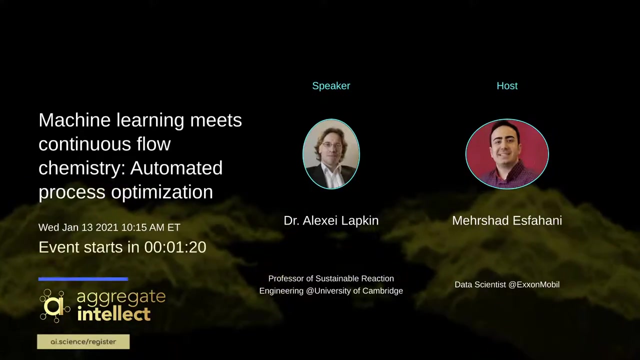 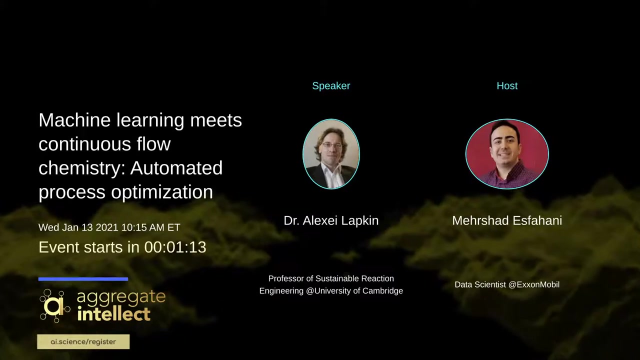 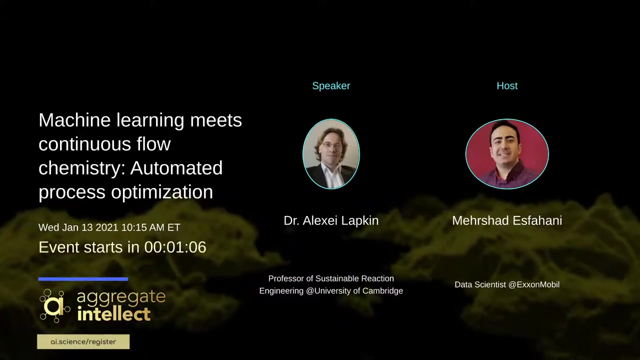 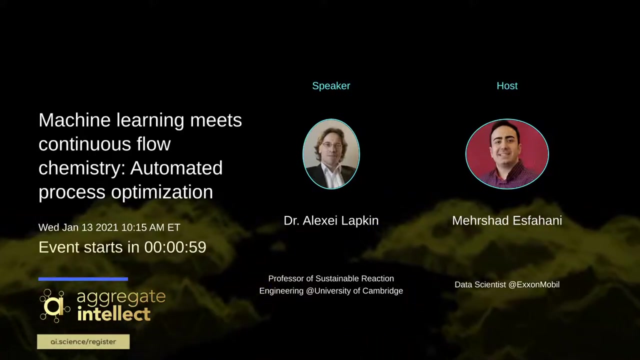 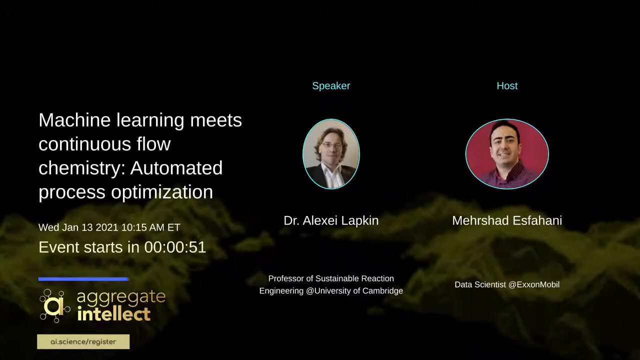 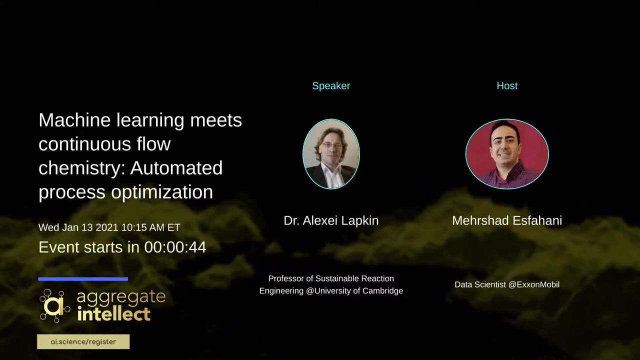 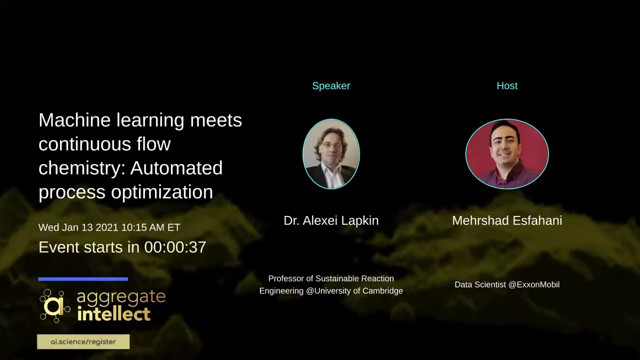 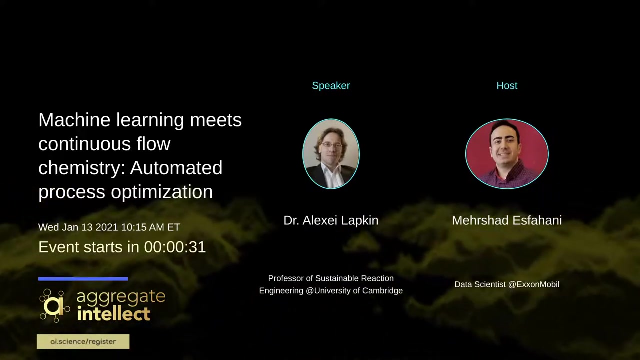 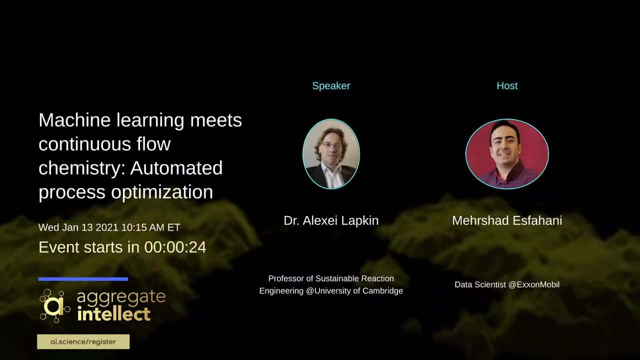 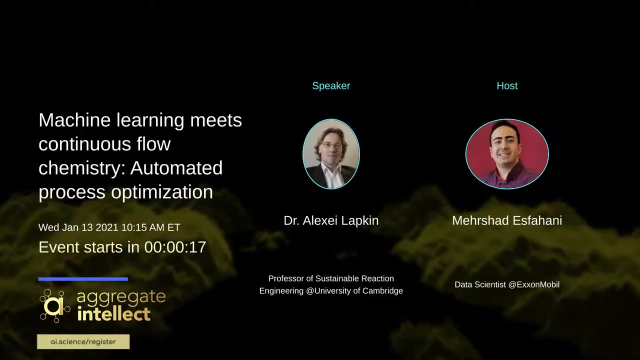 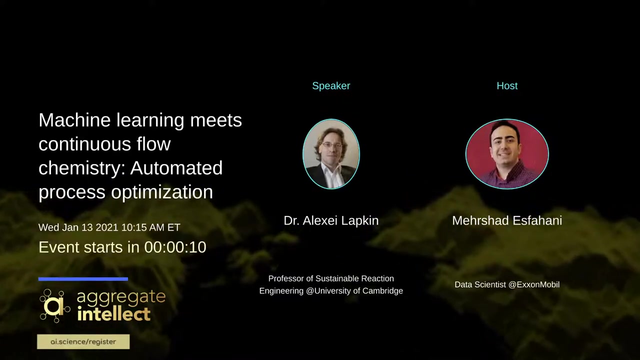 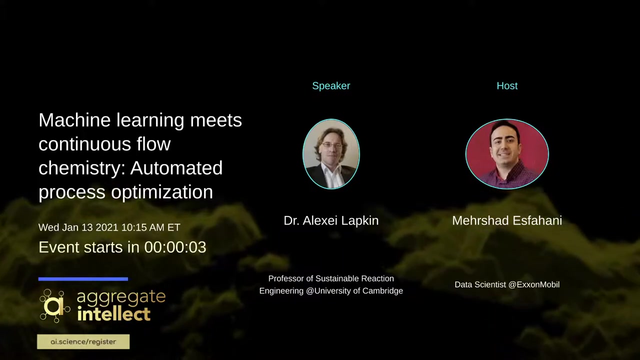 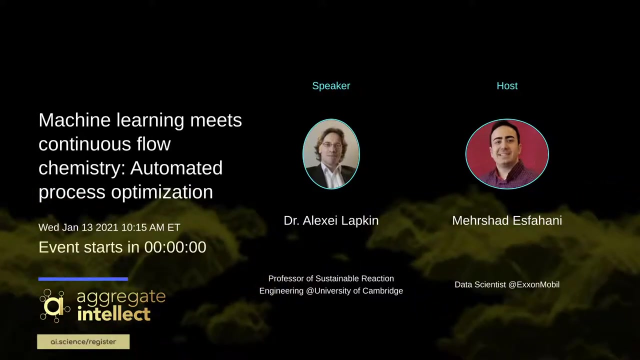 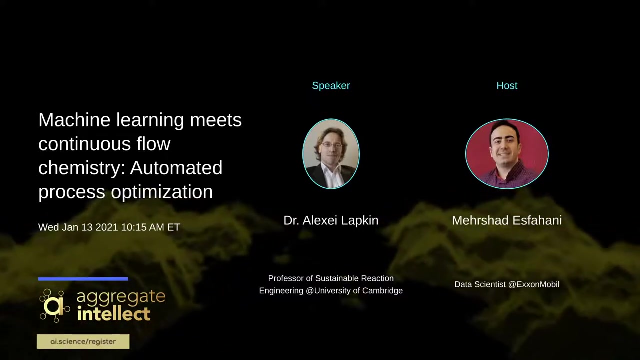 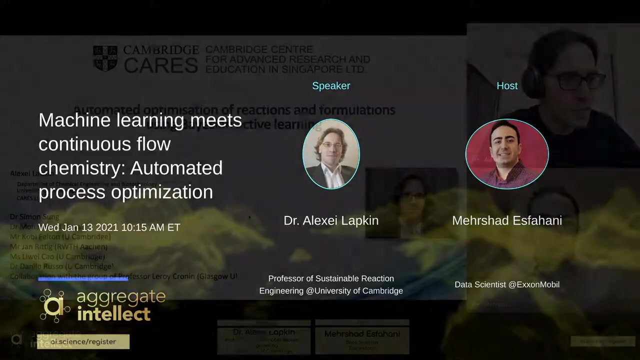 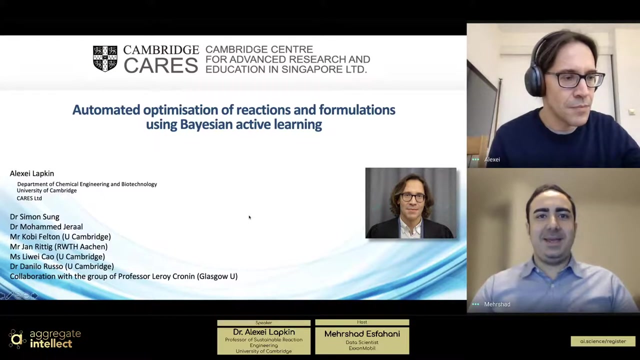 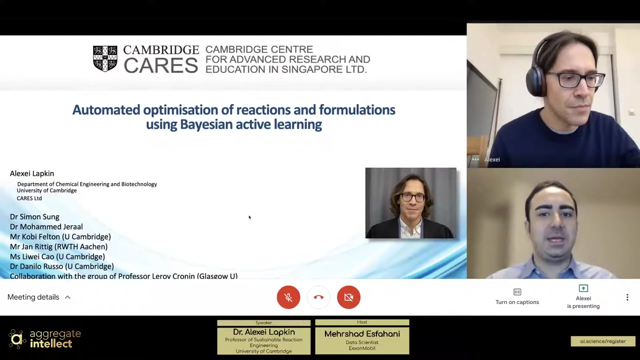 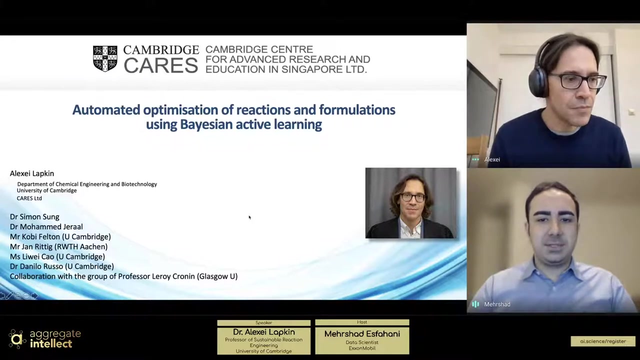 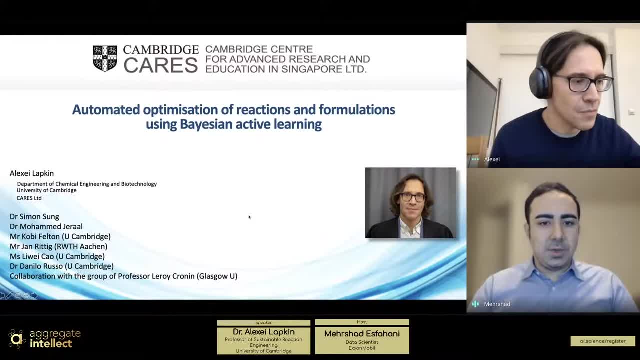 that have gathered around topics like AI research, engineering and products, And we host usually free live sessions, like three to five times a week, with a variety of objects. If you're interested, you can always visit aiscience website to get all of those talks and get to know more about the ACE. 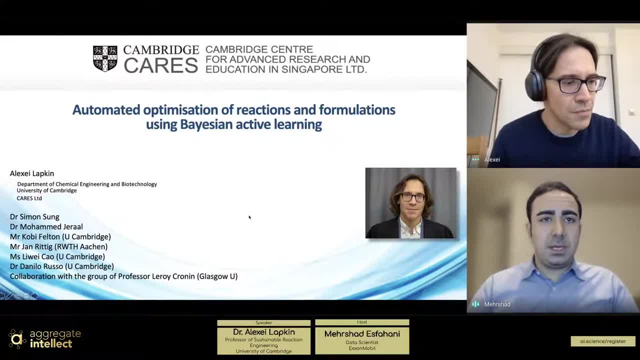 Also make sure you subscribe to the YouTube channel so you can get ML papers explained, You can get more talks like this in the future And also you can have access to the collection of the videos that we have already recorded. We currently have many stream owners focused on various ML topics. 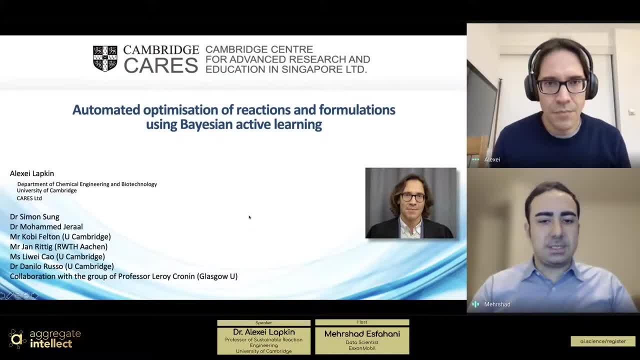 And this is ML in chemistry and chemical process stream. So I hope you enjoy this talk. Today. our guest is Dr Alex Dilapkin, And it is a great pleasure to have him as speaker. He got his chemistry degree from Novosibirsk State University in Russia. 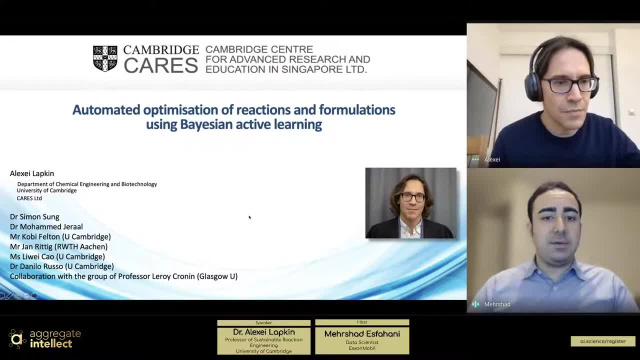 chemical engineering PhD from University of Balfe in the field of Catholic reaction engineering, And then he got academic position in chemical engineering in the same university since 2000 and appointed full professor of chemical engineering at the University of Warwick in 2009 and elected to the current position of professor of sustainable reaction engineering at Cambridge. 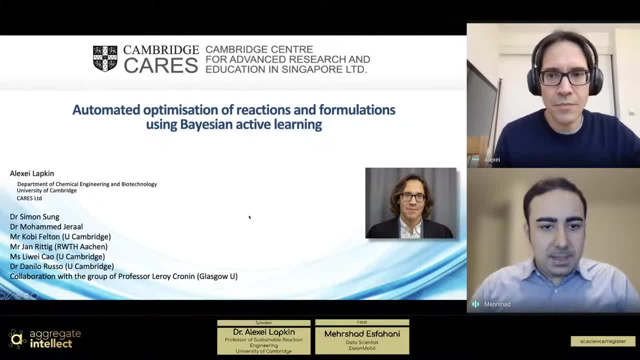 And he is now. he has several jobs, including being a director of innovation center in digital molecular technologies and deputy director of center for doctoral studies, And he is going to give us a talk about combining physical models with machine learning and mechanical engineering. And he is going to give us a talk about combining physical models with machine learning and robotic technology. 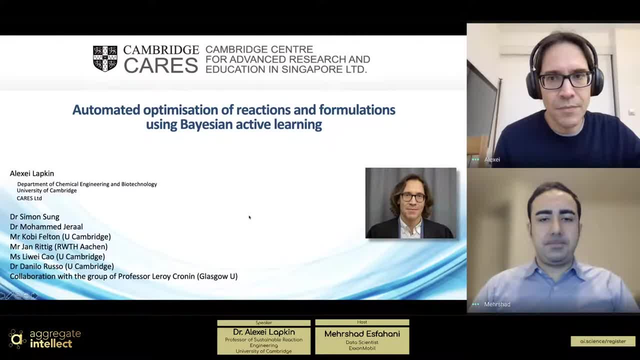 to develop complex chemical processes. Okay, thanks again, Dr Lockett, And we can't wait to hear from you. Thank you very much for the introduction and for the invitation to talk. As you see, I've changed my title a little bit. 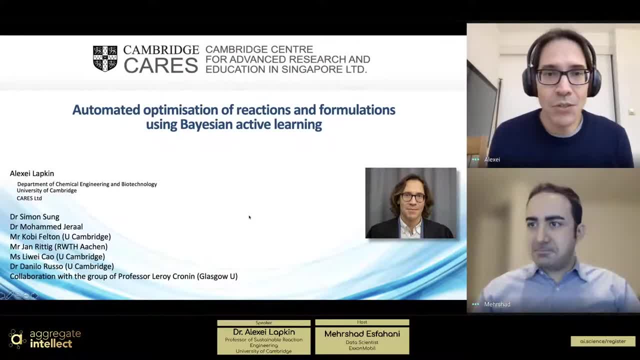 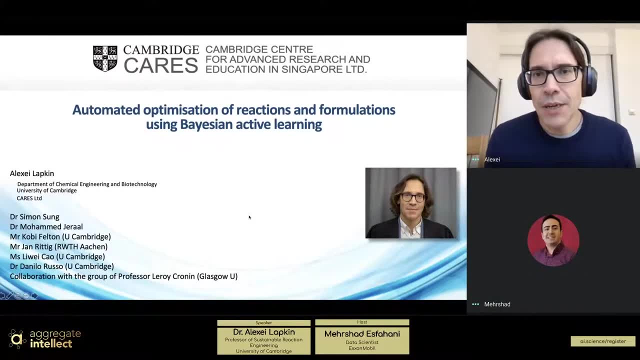 So I'm going to talk about the same topic. I'll just reformulate the title a little bit. It's the work. the majority of this work is done in our Singapore-based research center. It's called Cambridge Center for Advanced Research and Education in Singapore. 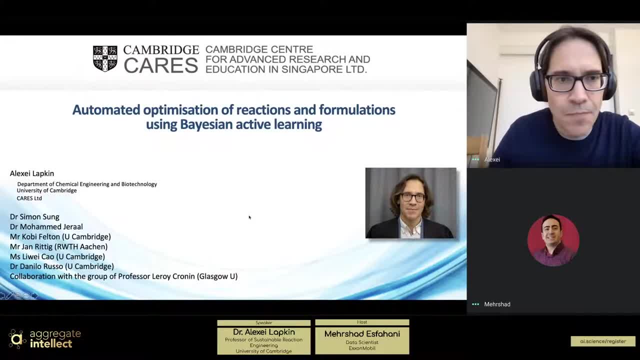 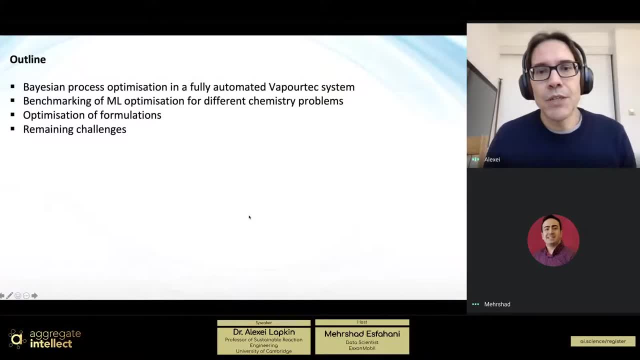 And part of this work is done in our lab in Cambridge. So what I will talk about is how to use, or why do we use, Bayesian process optimization in automated chemical systems. how we set up a system to benchmark different machine learning optimizations for specific chemistry problems. 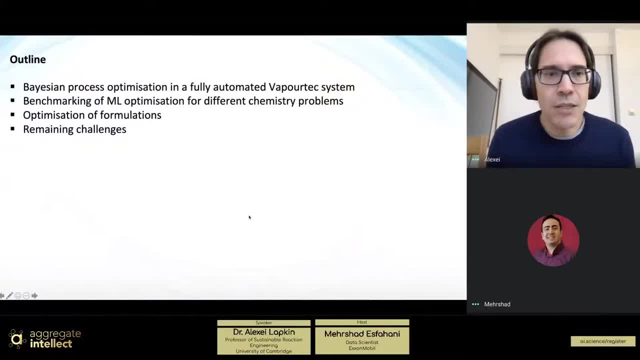 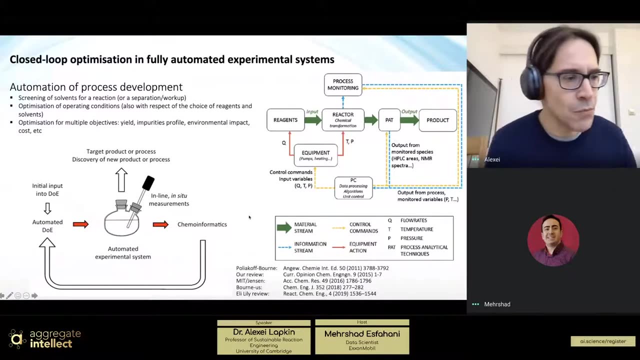 how we then use similar techniques in optimization of formulations, and then a little bit at the end about what I think are the remaining challenge for machine learning and for the whole field of digitalizing chemistry. So first of all, what do I mean by optimization of processes? 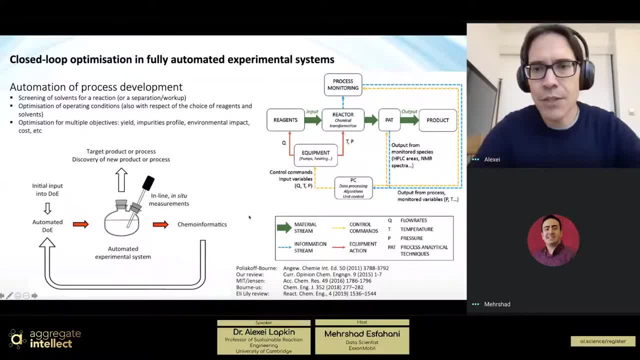 And why do we use machine learning? Where does it sit in the process development cycle? for us, I'm talking about the process development cycle, So we're talking about manufacturing and optimization of processes and optimization of products, rather than about discovery, And in this workflow, what we are trying to do is to increase the speeds of arriving. 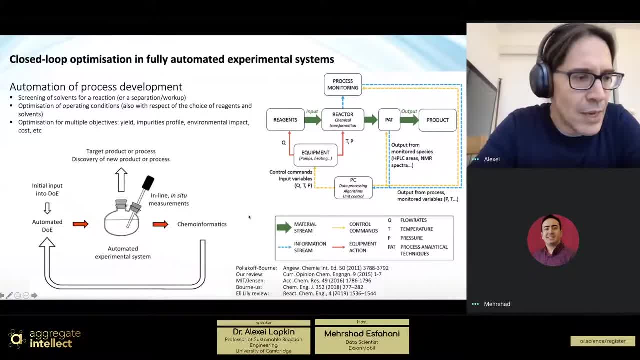 at a scalable, manufacturable process when all of the parameters for the process are optimized, Including Continuous variables and discrete variables. This field is now about 10 years old. The first paper I know about this field is from the group of Martin Poliakoff. 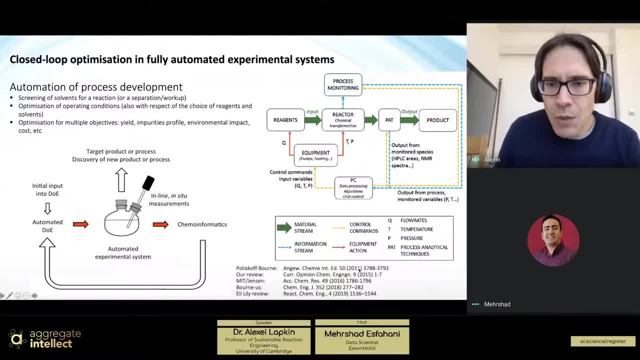 which was published in 2011.. Then there were a few reviews about this topic. Our review is now six years old from 2015.. Perhaps the best one I like is the review from Eli Lilly- This is in 2019 in reaction chemistry and engineering. 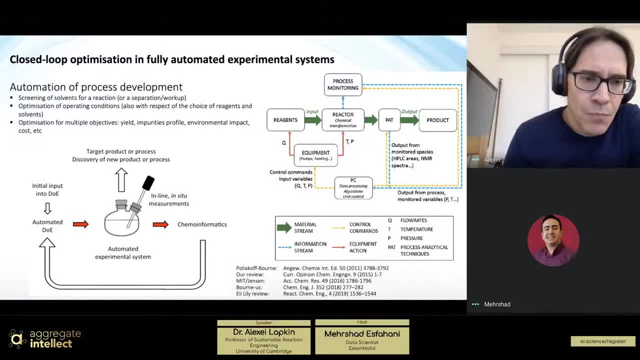 So in this automated process optimization, you have a number of components. You have an experiment which is a reactor which needs to be fully automated. It takes measurements, It performs the reactions, It performs separations. The measurements are then converted into something meaningful using chemoinformatics. so we understand. 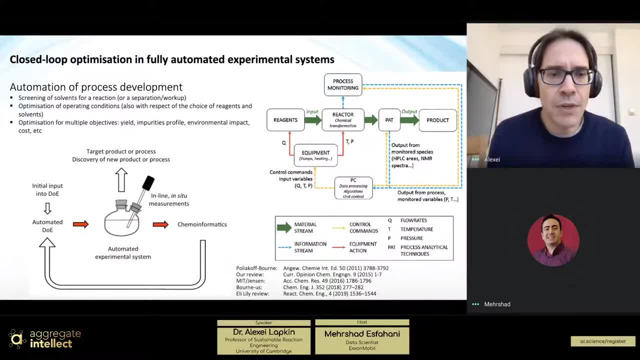 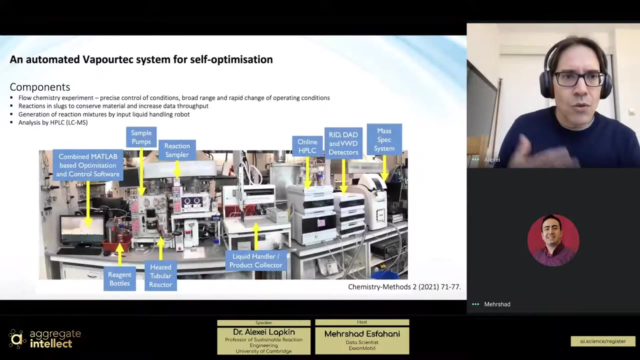 what have the system achieved Then? on the basis of these experimental observations, we need to create new hypotheses about the next experiments to perform. So this is where active learning comes into play, And this is where we need a brain and where the machine learning algorithms come in. 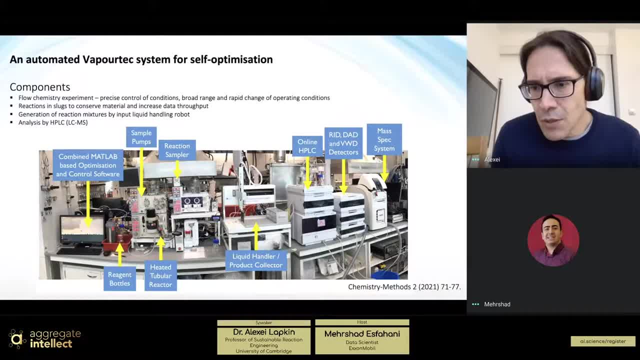 So this is our current system. It's recently been published in the New York Times. It's a very interesting system. It's a new journal from Wiley Chemistry Methods. It consists of a commercial continuous flow chemistry setup. So the bits in the middle are the reactor modules and the pumping modules, which are 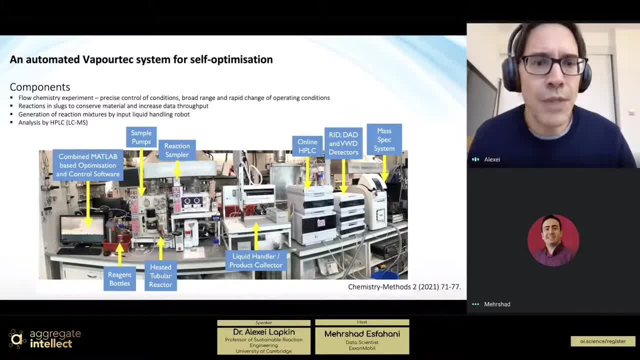 easily automatable because these commercial systems comes with an API. You can address all of the components and you can run it from pretty much any software you like. Okay, So how do you feed the system with designed experiments So you can choose the discrete variables? 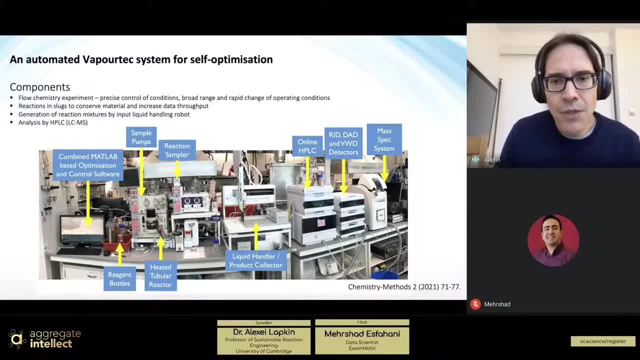 You can choose: reagents, solvents, catalysts. We put some of the components in reverse. So in this case we have a liquid handling robot which is typically used to collect the product fractions. We use it both to collect the product fraction but also to create the feed mixtures which 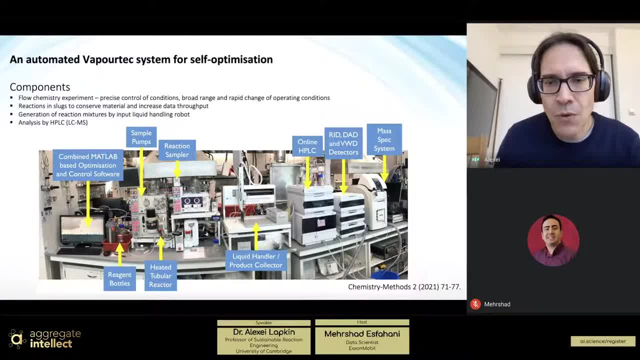 are fed into the reactor. So you set up your Okay Feed solutions in the rack and then program the robot to create the right mixtures based on the designed experiments and then those go into the reactor system. We perform the reactions in flow, but we perform them in droplets so that we don't waste expensive. 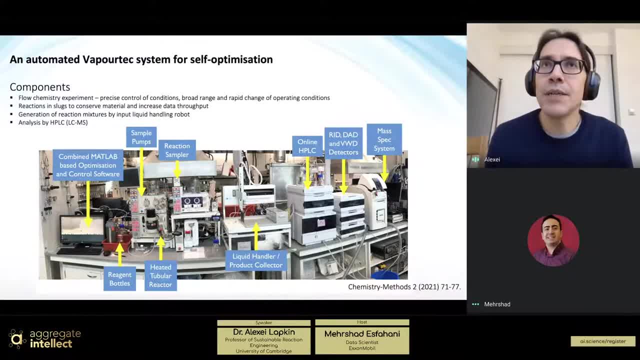 reagents. The size of the droplet is limited by dispersion in the pipe. If the dispersion is too high, you cannot have very small droplets, So you typically have those quite large slugs. Okay, So they are in a pipe and the slug volume is about three milliliters or so. 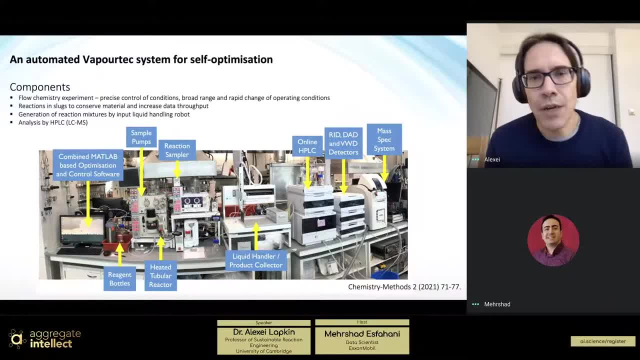 If you go a little bit smaller then you might have the effect of dispersion on the results. To analyze the results, we have an online HPLC instrument and, if you want to, you can also call it with the mass spec. Some other people have coupled this with infrared or with even inline NMR. 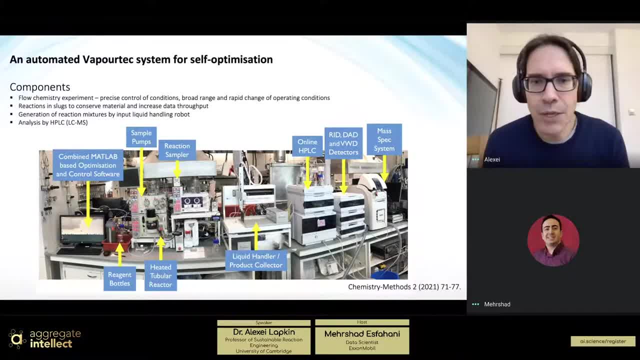 Okay, So all of these things are entirely possible. That depends on your budget and on the specific chemistry problem you want to study. So the entire system is connected to one system which runs the whole thing, which programs everything, times the analysis and runs the machine. 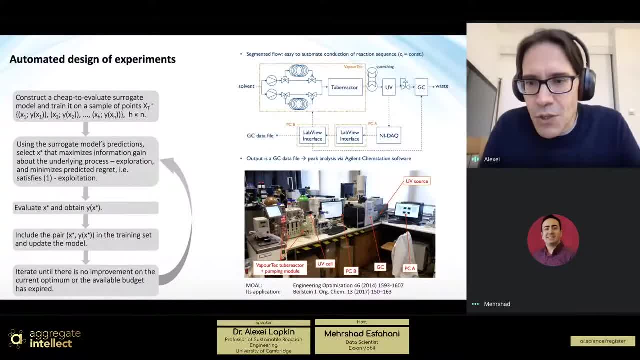 So this is our current iteration On this slide. I'll show you. Okay, So this is the iteration of the same thing, which is in our old lab. It looks much more rugged than the newer boxes, but it still worked. We published it a few years ago. 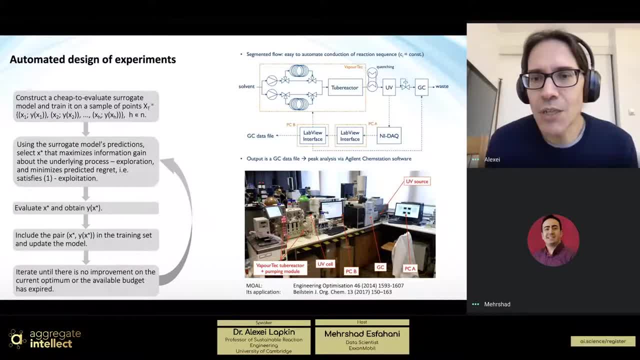 It's a very similar design, again the same VaporTech machine. similar, again sampling from line, but in this case using GC. and we used a very, I would say, genuine way of running the GC by basically programming A mouse to click the run instead of doing anything else. that was the cheapest way of 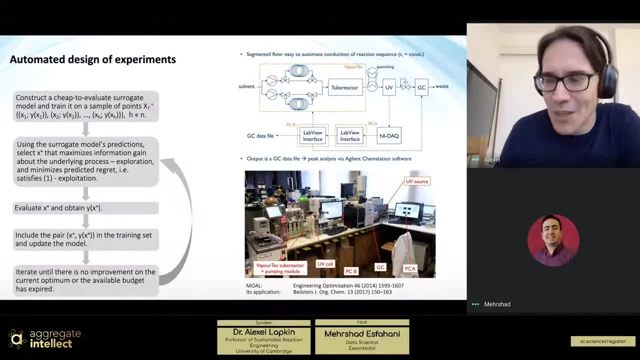 doing automation, in this case very much student led project. So to run this we use Bayesian optimization. We use algorithms which construct a surrogate function which estimate what's going to be the outcome. We then try to minimize the uncertainty of the model and target the regions of the experiment. 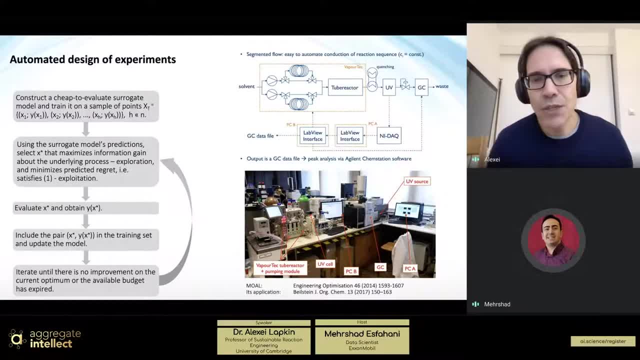 So this is the standard way of running this type of optimization problems. We use Gaussian processes typically. they're very good for chemistry. They work in most of the cases. They work with sparse data sets. They don't require a lot of data and, besides, the fact that we can have the uncertainty- 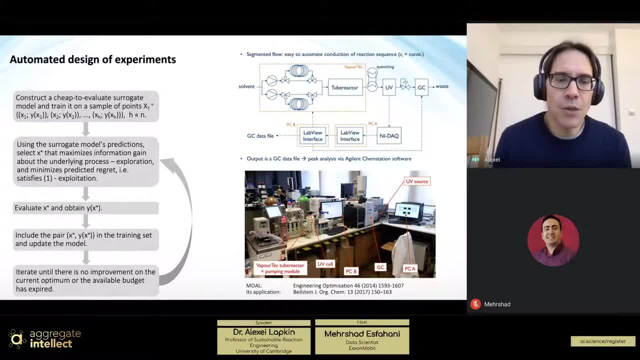 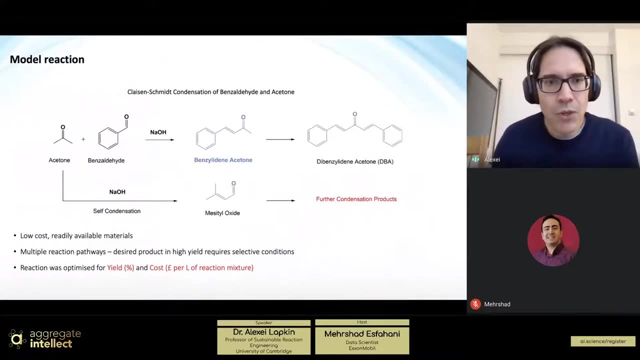 the surrogate model explicitly helps in designing the workflow for active learning. So that's the reason why in many of the studies of this type, people use Gaussian processes as a surrogate model. We use this chemistry as an example. We don't need to go into detail. what it is. 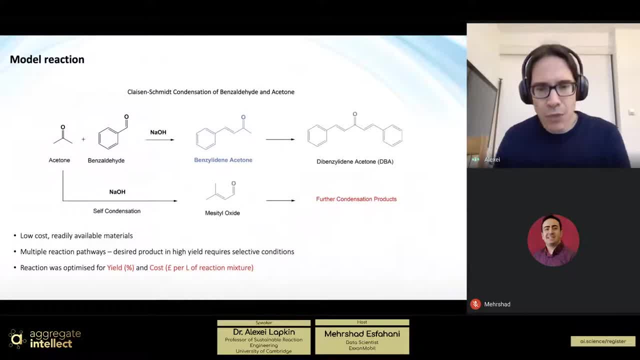 The only thing which is important. there are several outcomes which depend on the process conditions. So you change the process conditions, outcome, And then the system is nonlinear and you have a number of possible targets. You can target the minimum cost, You can also target the maximum yield, for example, And the results are: 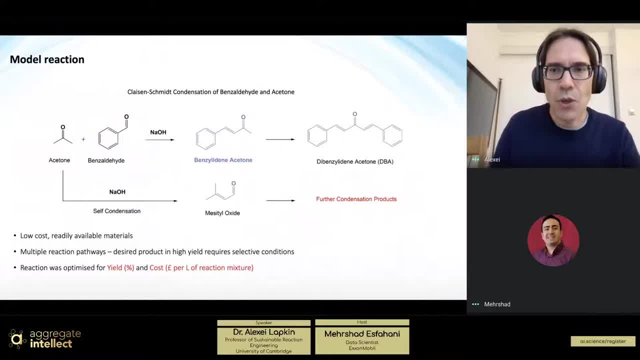 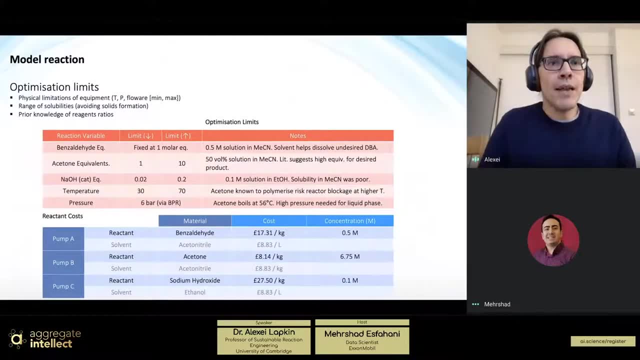 not necessarily the same. So the system is a nonlinear system. In order to set up any automated system, you need to give it limits. And this is the question we always get asked: How do we set it up? Can the system run entirely autonomously, Or you require some kind of 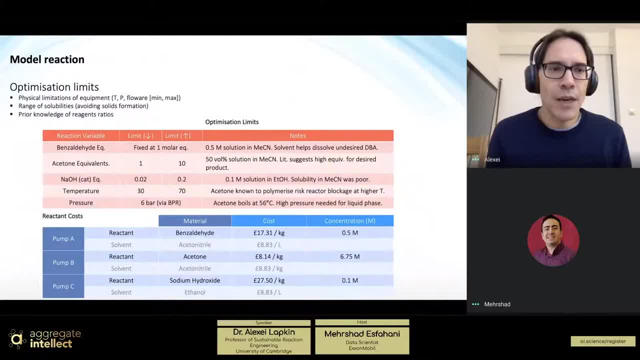 knowledge from experts And yes, of course you do require some knowledge. You need to make sure that the system runs within its physical limits in terms of temperature, pressure, flow rates of the system. But then also we run this in flow, which means that we're limited by running everything in liquid. 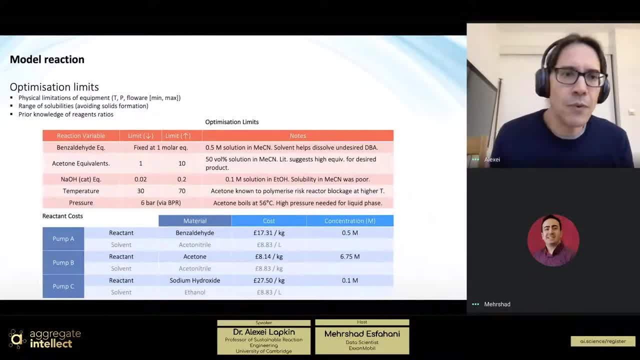 form. We try to avoid solids due to the type of equipment we use. If you change the equipment, you can do exactly the same using different setups which can handle solids, And in this case you're not that limited by the range of solubilities. We also use prior chemical knowledge, So we use 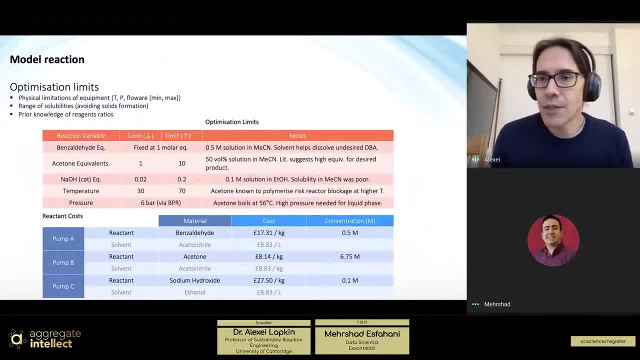 knowledge on, let's say, ratio of reagents. And in one of the examples which I show you, we also use a prior model before we do optimization, But we'll come to that a little bit later. So we have our tables with the optimization. 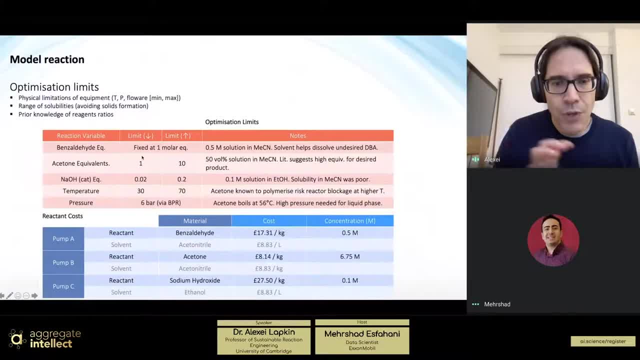 limits. We set also the ratios of reagents which we know make sense. So it doesn't make sense to go outside of those. It's not going to work at all. And we also give the system the knowledge of the costs of the reagents. So that's how we calculate the minimum cost of the process. 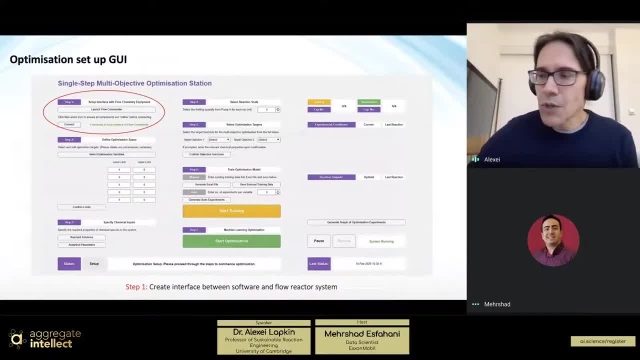 Now I presume I'm talking predominantly with people who understand machine learning. However, the users of our methodology are people who typically understand chemistry. So in order to combine those two, we've created a user interface, And I'm not going to go into. 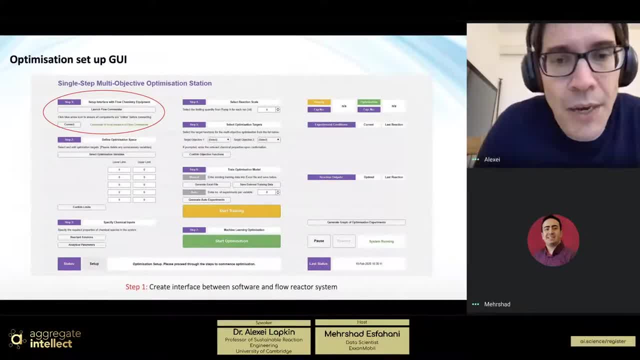 which actually speaks to chemists with the language they understand. So any experienced chemist could come up to this machine and actually set up an experiment without having to do any programming themselves. It's all done at the back. So it starts with the launching the connection. 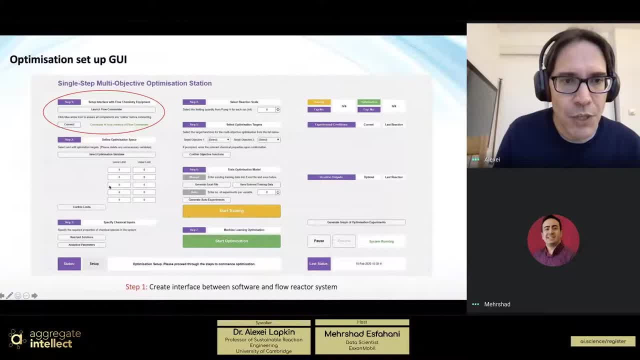 to the flow experiments, then define an optimization space- What do you actually optimize and what are the limits for those? Then looking at the analytical parameters for the system, then selecting the scale. So how? what's the size of the droplet you're using? 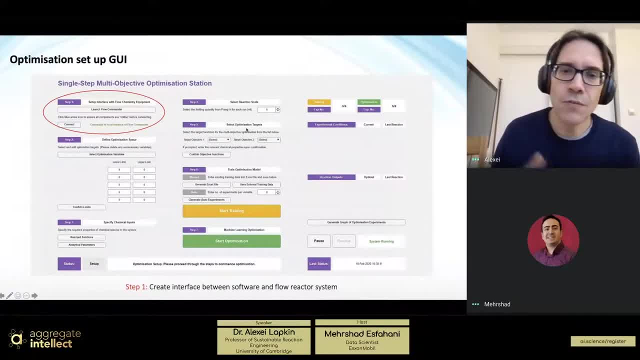 Then looking at: okay, what do you actually gonna optimize? Are you gonna optimize for yield, for selectivity, for environmental impact, for cost? Typically, we optimize for two targets simultaneously. You- we have now a version on this screen. it only allows you to select two. 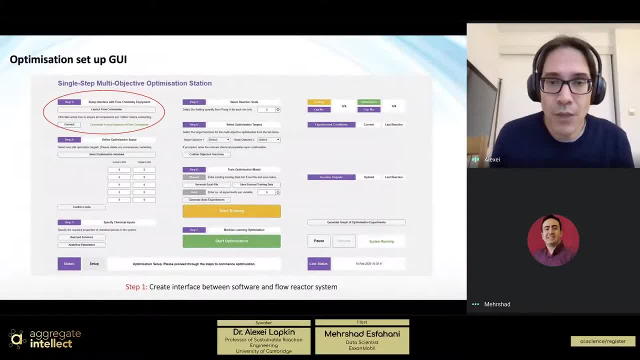 We have a version where you can select three or four simultaneous objectives and we use a multi-objective algorithm, which I mentioned. Then you can train the model. And this is you either use the data you already had and you just upload the Excel file. 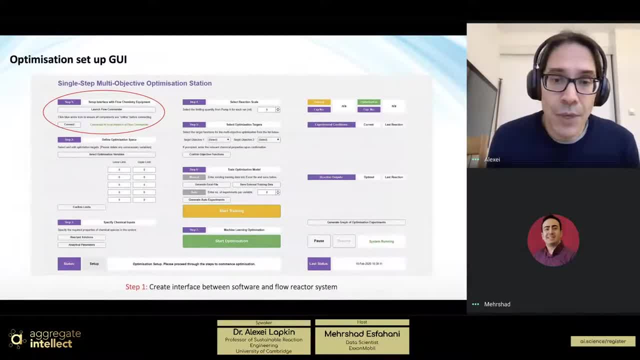 or you generate a prior And we use Latin Hypercube for that And you can use another initial design if you want. For some cases, if you're doing kinetic experiments, it's Latin Hypercube is not the best way. Typically Latin Hypercube works. 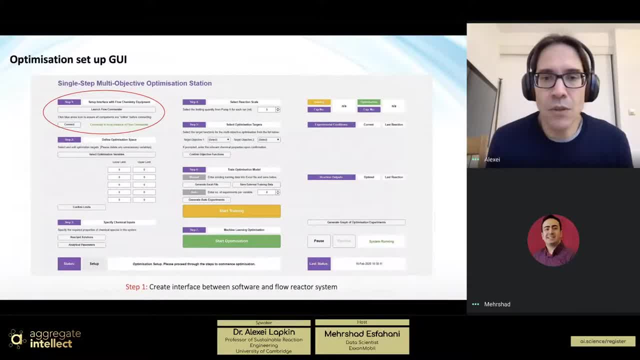 It's not always the most efficient prior, but it sort of the prior data set, training data set, but it seems to work okay. And then you start optimization and the system works. It also shows the current results, the past results. 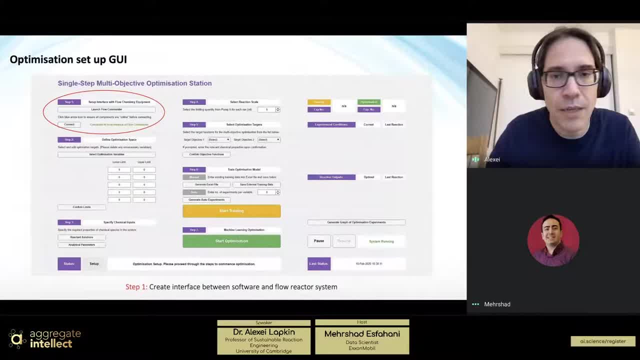 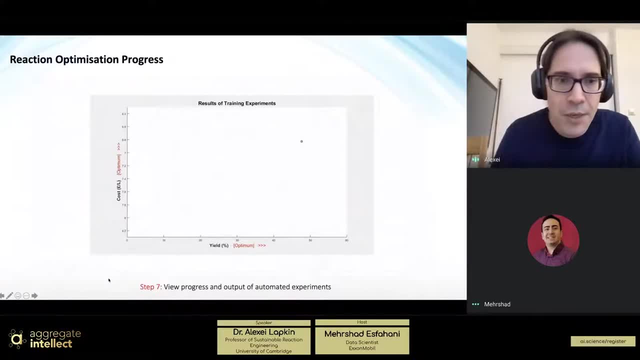 the current optimum And you can always get the data out and have a look at what's going on. So let me show how it works Here. we're optimizing for cost and yield, So we want the highest yield, which is on the right. 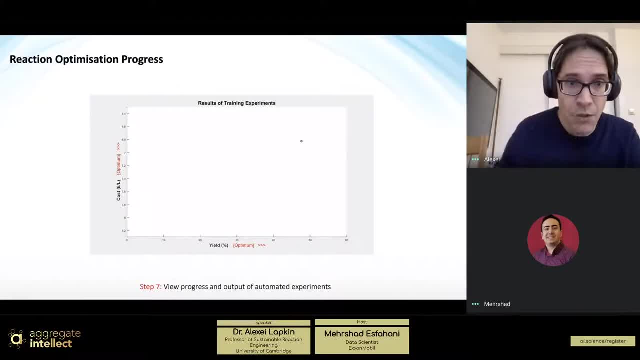 and we want the lowest cost, which is on the top. So the cost is in reverse in the axis. So the optimals will be on the right top corner And our training set is the circles and the optimization set is then will be the crosses. 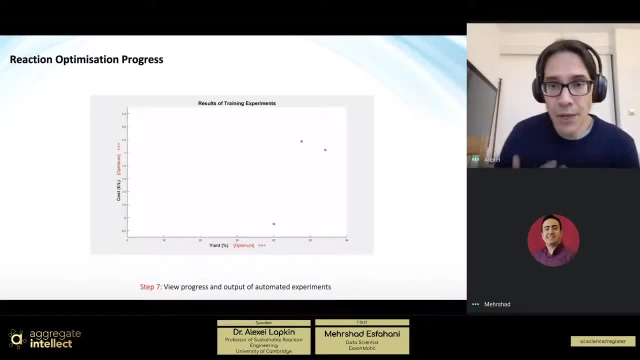 So initially we run the training experiments. This is like Latin Hypercube designed, and they obviously explore the space, So they are all over the space. And then you start running the actual optimization experiments, which are then congregating fairly close at where the optimal solutions are. 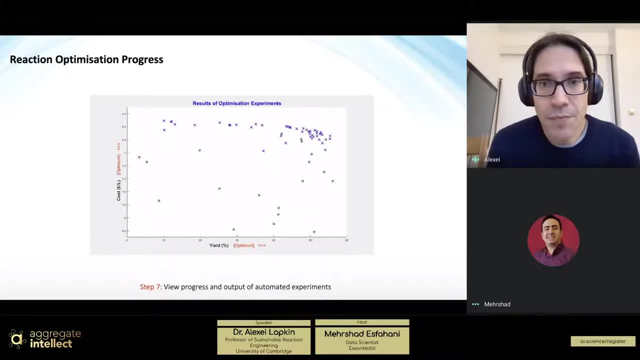 So, as you can see there, fairly densely concentrated at the top right, top right line, top line and top right corner. so this line is the set of parita optimal solutions. so all of the solutions there are correct, they're all optimal and you just need to choose the one you like. so you obviously you're. 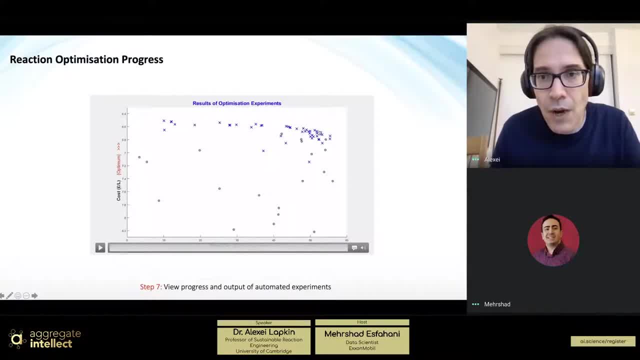 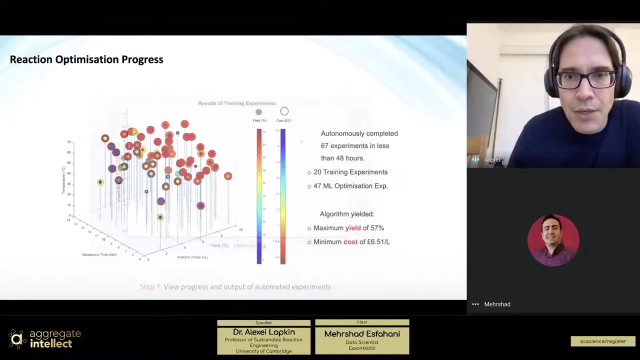 going to choose somewhere something a bit further to the right where you have high yield, because the costs don't vary that much. so somewhere there you would have the uh, the solutions, uh, you would want to pick. so this is how this works. so this was done in uh 67 experiments. they were run by the machine. 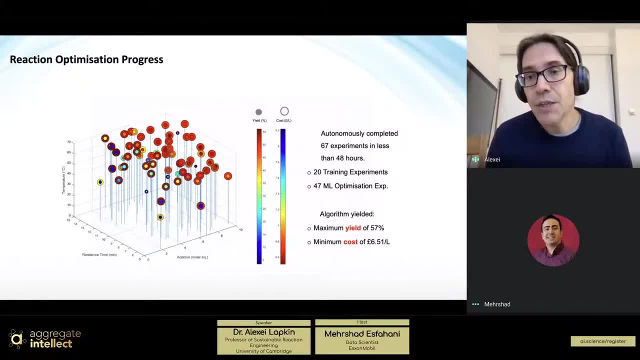 without, uh, any interference. so 20 training experiments and then 47 optimization experiments were really all good as well. so this is actually a rather complicated infographic is really for people. if you really want to see that the system is non-linear, then you can see it here. that there. 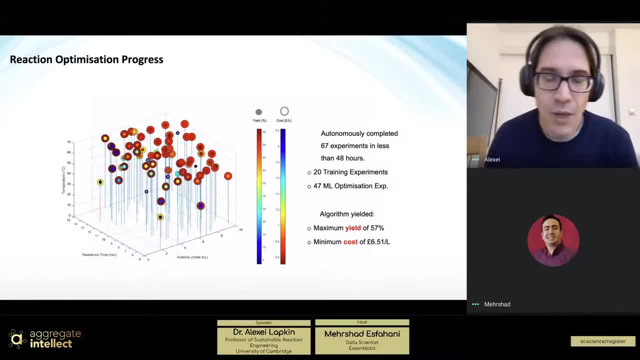 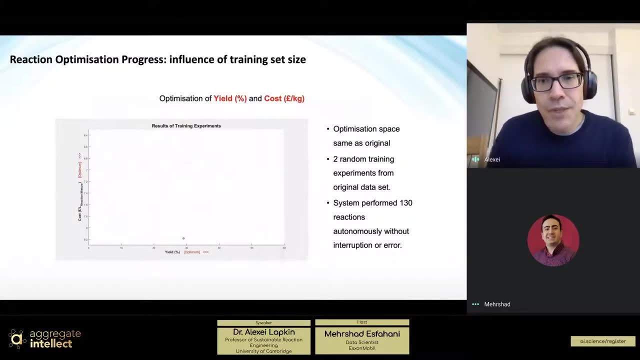 are data points. where the yield is high, the cost is not optimal, and vice versa. when the yield is low and the cost is is low, is low as well. so it's it's not not a linear system which is easy to. So, out of curiosity, the researchers who built the system and did this work, Simon and Mohammed- decided to break it. 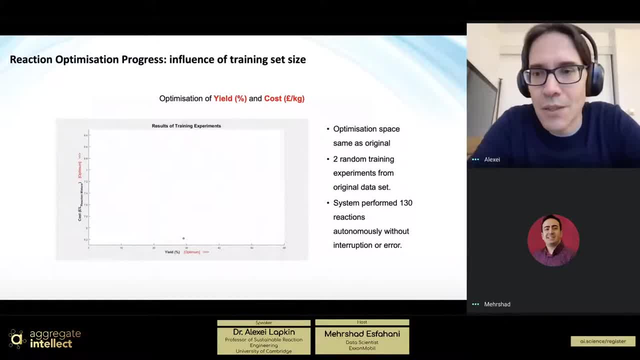 Well, they didn't write the algorithm, They put together the whole system, And so they decided to give it very, very little training data. So instead of 20 data points for latent hypercube, they gave it two and decided: OK, how is it going to fare? 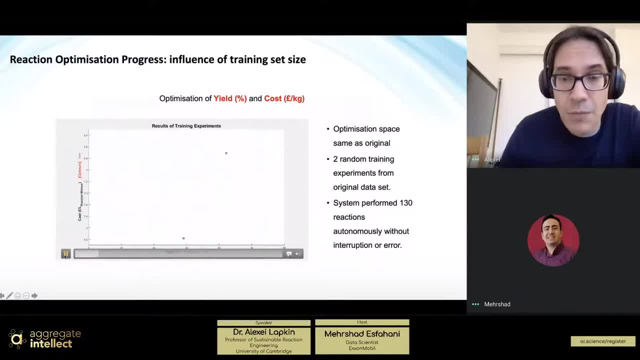 And they run it for 130 total experiments. So these are the first two data points. They're in the middle of the yields, But those are actually recent yields for this reaction at different costs. And then the TSEMAR algorithm we are using actually have to explore a lot more. 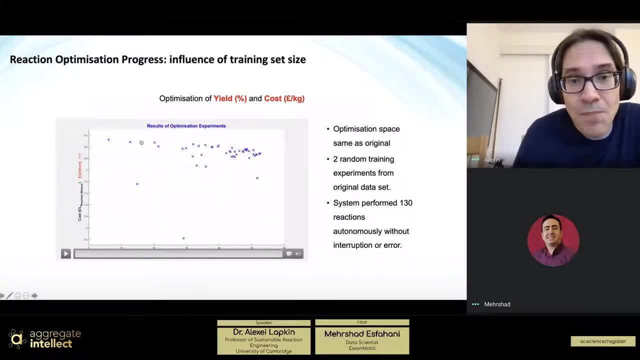 In fact, the TSEMAR algorithm we are using actually have to explore a lot more in order to get to the right set of solutions, And it does actually fare reasonably well. It still finds quite a lot of data. It's not as dense as before, but it's not bad at all. 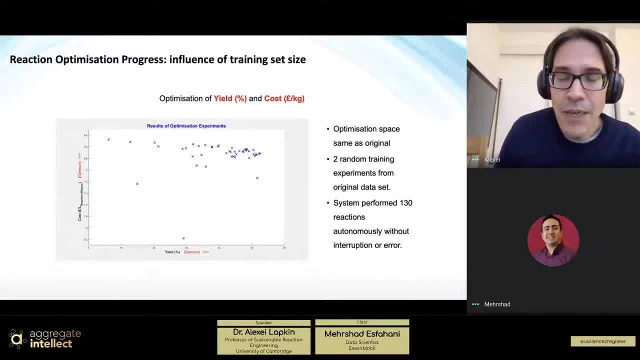 So then they were encouraged by the fact that they couldn't break it. So they decided, instead of giving it the yields which are already reasonably good, try to give two data points which are really very bad. So they decided, OK, I'm going to break it. 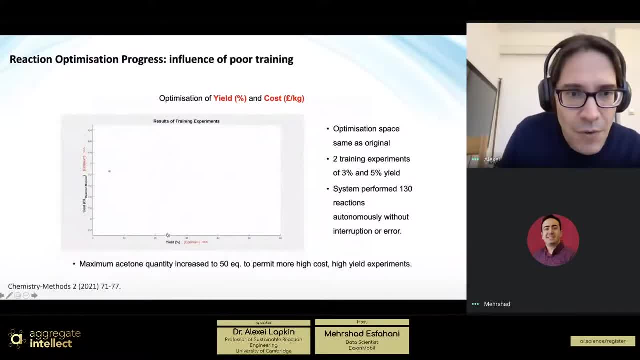 So they decided to give data points which are very low. So in this case the yields are very low. So this is the first one, Then that's the second one again, And then, of course, the system is very. the algorithm doesn't have any data about where the right solutions are. 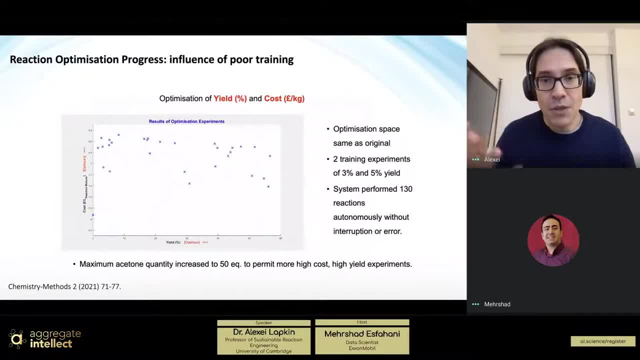 So the exploration then takes longer. So the data points go all over the place And still in the late optimization runs you see that it begins to concentrate around the Pareto set of solutions somewhere in the top. So what is encouraging for us is, at this stage in the state of the art of the automated optimization, 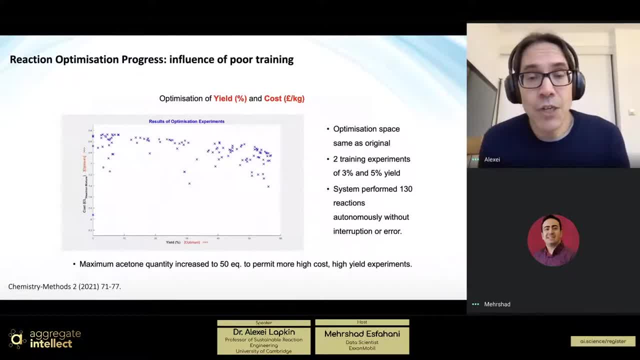 you can pick a now off the shelf algorithm. We are using TSEmo, which has been adopted by a few groups. It's open access. You can download it. You can re-implement it. We've re-implemented from MATLAB into Python and automate the commercial equipment using fairly standard automation setup. 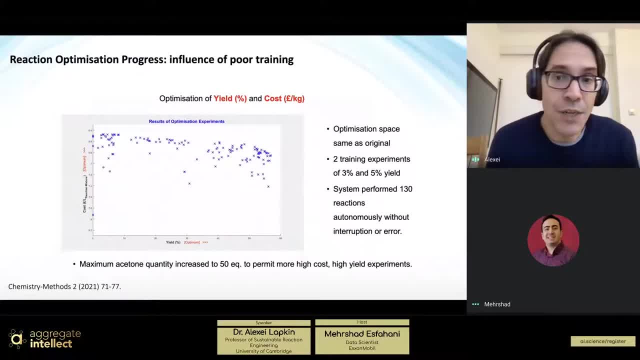 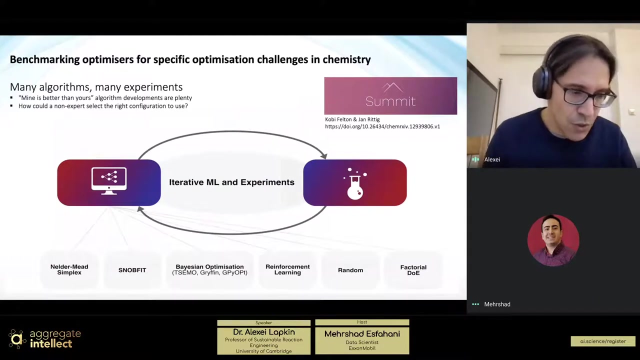 Everything is automated for LabVIEW and run experiments- In this case, 130 experiments. It's several days of work, It's almost a week And the machine works on its own. It only will send an error message If something is wrong, like a pub stopped or the solution bottle ran out of solution. 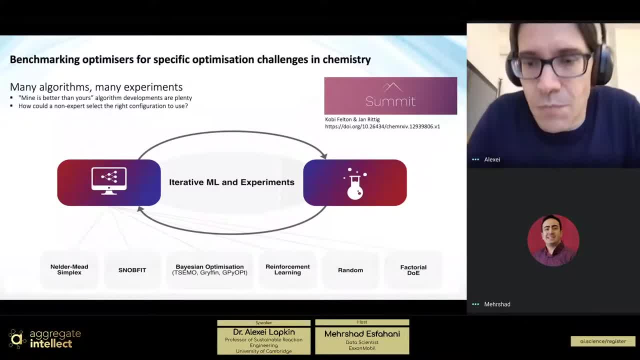 Now, in order to understand which algorithm to actually use, my group decided to look at standard types of problems which many chemists or process chemists face and then look at the number of algorithms out there and see, OK, can we develop a tool which helps users to understand what's the best algorithm for a specific problem? 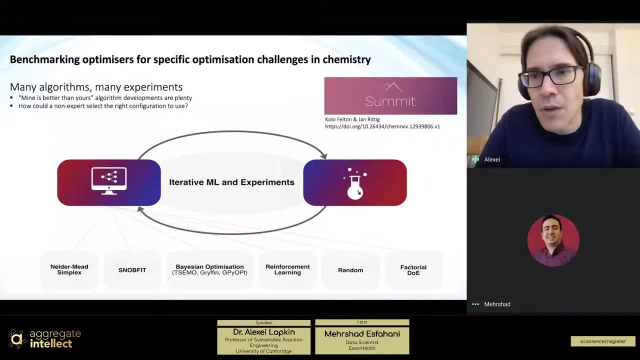 So called benchmarking problem. They've set up this code which is called Summit. It's again. it's on GitHub. It's open. The review, the chem archive paper is out and the peer reviewed paper is already in production. It will come out in the same chemistry methods journal quite soon. 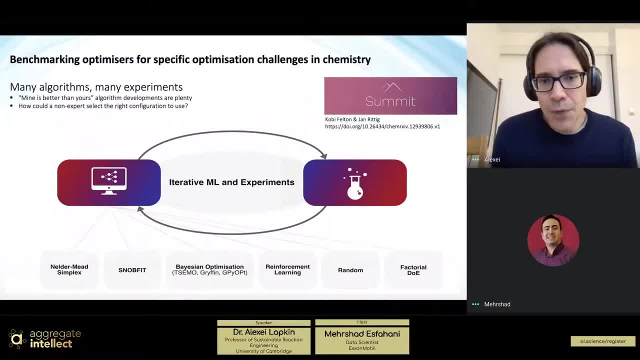 So what this system does? it picks an algorithm which the user chooses to try. It has a set of standard problems which are already encoded, based on physical models as well as based on machine learning models, and then runs the algorithm, Runs the optimization, compares the different algorithms in several metrics. 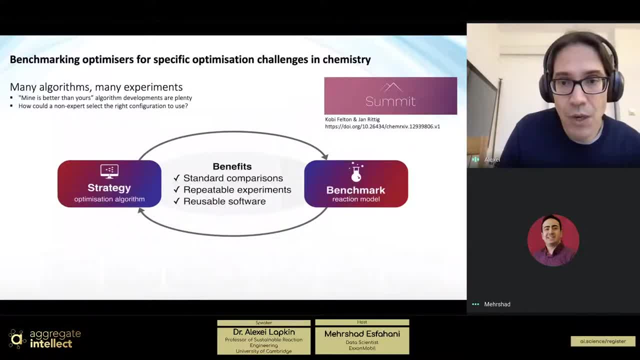 and then gives you the comparison. So let's just see how it works, So you can upload your own experimental data for this and your own chemical system and then try to run it to see how well a particular machine learning strategy works for this. 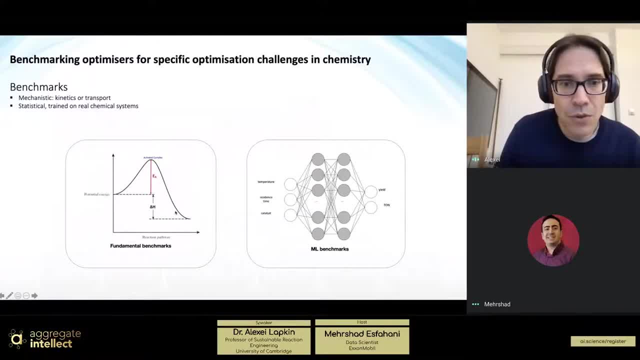 The mechanistic models which can be used are basically differential equations, So they would be continuous functions typically, And if you have a machine learning representation then it would be some kind of surrogate which represents the real system. So if we look at an example, this is the literature example. 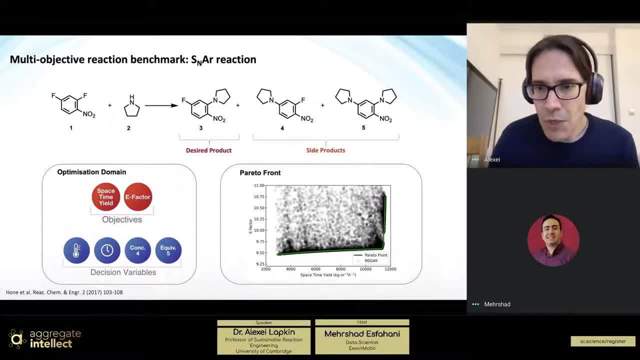 which has a machine learning model behind it. So there is a known data set. It's a multi-objective optimization. Again, you have space, time yield and environmental factors objective. You have four decision variables and four types of decision variables. 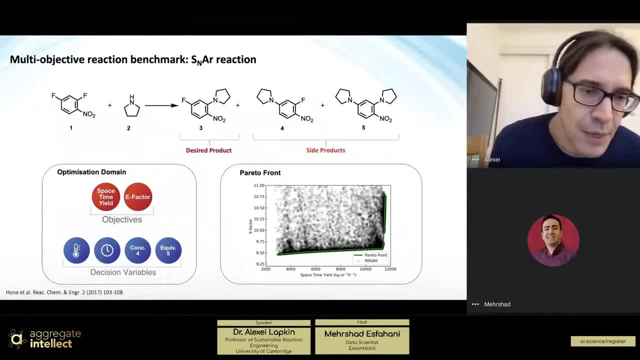 Concentration for concentrations, equivalence, time and temperature, And you see how dense is the data set. It's actually quite a lot of data. So there is a neural network which is behind this tool. It's a neural network which is behind this reaction as a surrogate. 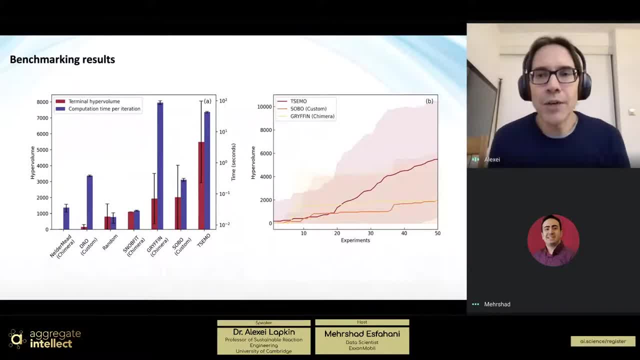 And then, once you run the comparison, the benchmarking, in this specific case, the TSEmo algorithm seems to be better. So you see that it reaches the highest hypervolume in the smallest number of experiments on the right-hand side. So the larger is the hypervolume, the better is the model. 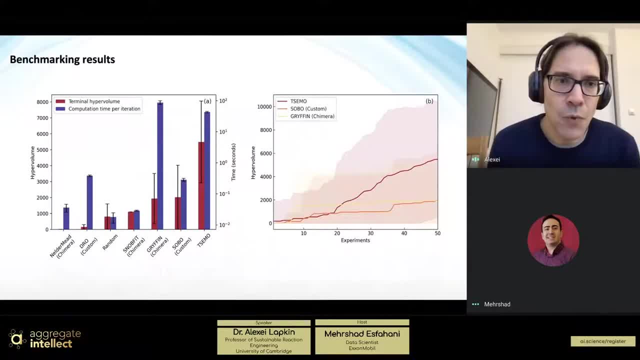 But if you look at the comparison with also the computational time TSEmo algorithm in this left panel is the rightmost two bars. It's actually quite hungry with computational time. It's not the hungriest but it is quite hungry. 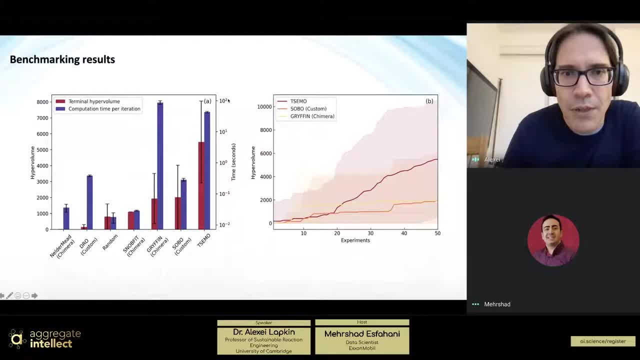 And so for some of the problems, you may not want to use such an algorithm. You may want to use an algorithm which may be not as accurate but also not as computationally expensive, And some algorithms are much worse. In this specific case, for example, Chimera have a low accuracy. 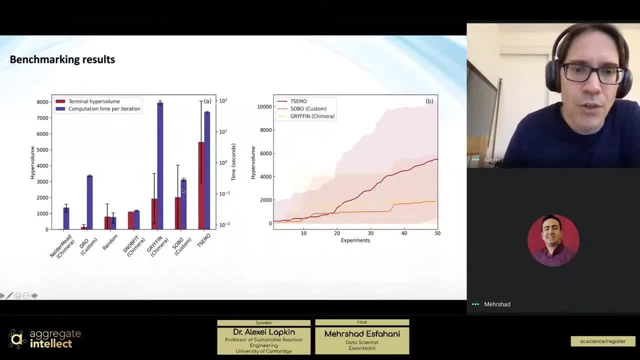 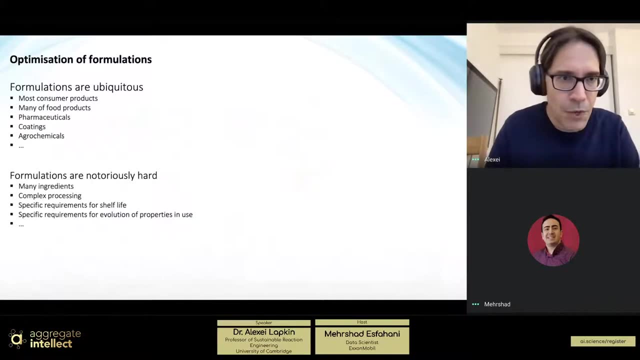 and high computational cost. Some others are not that bad. So we have other benchmarking studies when, on different cases, other algorithms are actually performing better than TSEmo. So it's the tool which allows to do this comparison. In the last part of the talk, 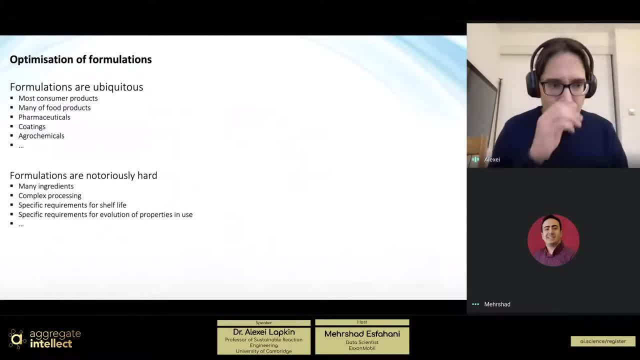 and I actually have about three minutes left for what I gave myself, but I'll probably take a little bit more. I wanted to talk about how we use similar approach to optimize formulations. Just to say what are the formulations? Formulations are complex mixtures of ingredients. 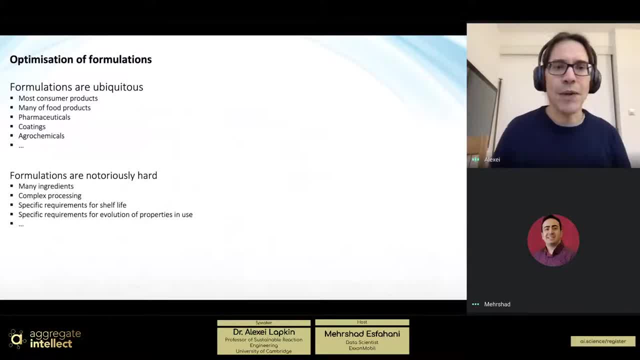 Your shampoos, lots of other consumer products, many of the foods, pharmaceuticals, coatings, agrochemicals- all of those are formulations. They have many ingredients. They require complex processing, They have specific requirements for shelf life. They have specific requirements for evolution of the properties in their use. 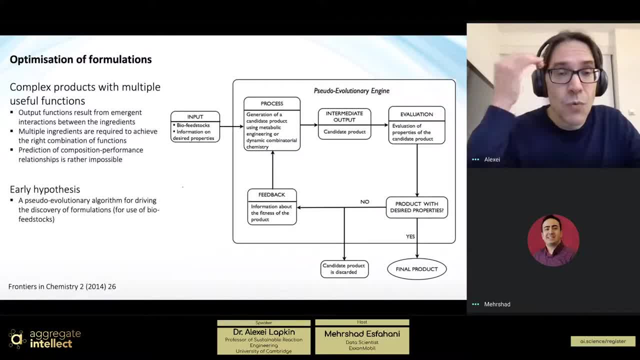 If you think about shampoo, for example, We thought about using some kind of evolutionary approach to design and fabrication of formulations quite a while back, So we published this concept paper about how we would possibly do it from Biofeedstock a while ago. 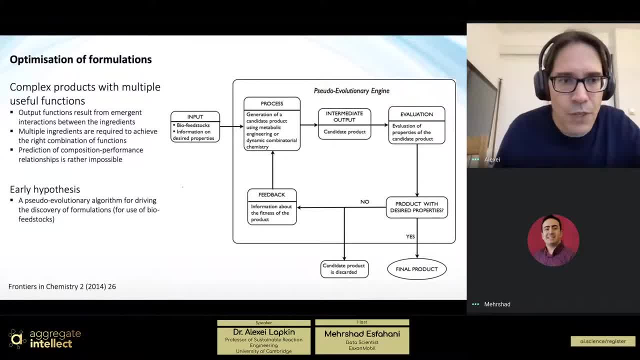 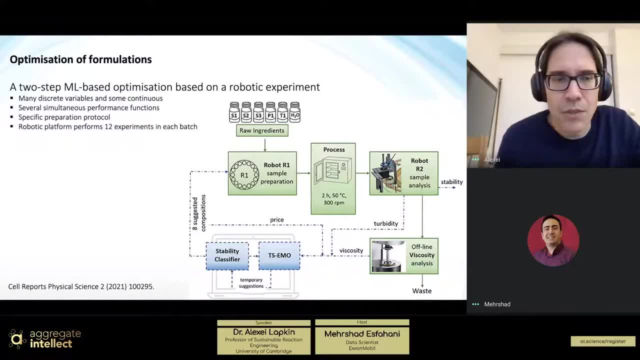 But we couldn't do it. We didn't have enough tools for that seven years ago. So this is the new tool which we've just published. The paper came out just a couple of weeks ago. What it does, it takes a robotic system. 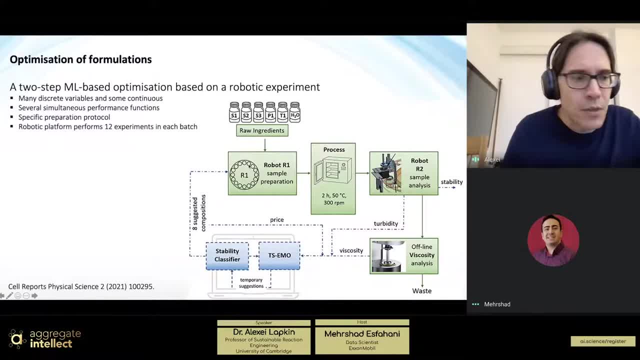 which can make the formulations. It uses two algorithms. One is a classifier which is trained or pre-trained on some data And it basically says: is your formulation you're going to make going to be stable or unstable, And you want a stable formulation. 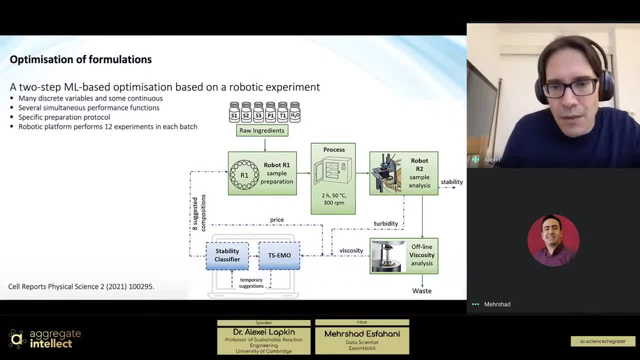 so it's stable in use. And then the second part is the regression model, which is, again we use TS-SIMR, where we then optimize in the composition to get the right viscosity and also the lowest price. So in this case we actually have three targets. 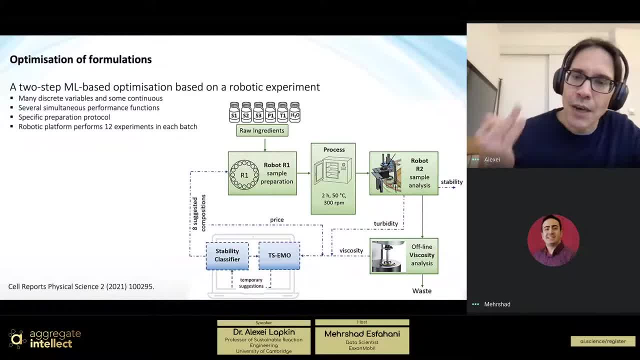 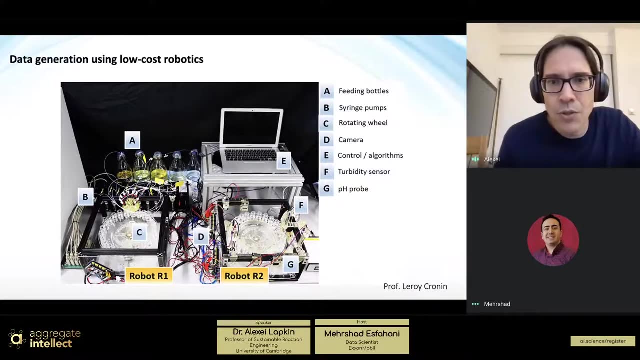 We want a stable formulation which has low price and has low viscosity, And then we run this whole thing as an optimization approach. So this is a collaboration with the group of Leroy Crone in Glasgow. They build low-cost chemical robots. 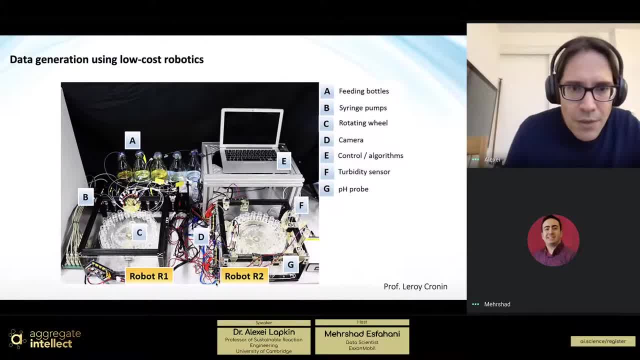 So this is the way how this robot looks. The left-hand side robot is the one which is making formulations, So it basically pumps which feed solutions in the right ratio into the vials. Then the robot we take the vials for processing. 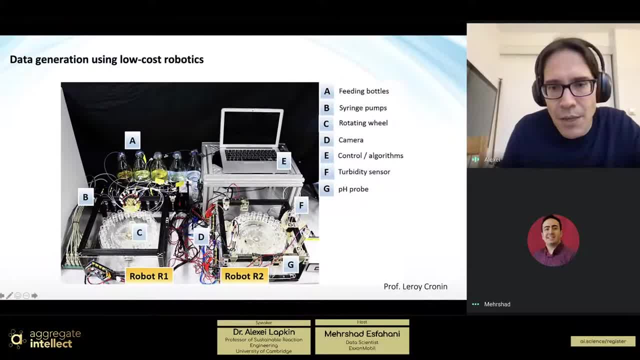 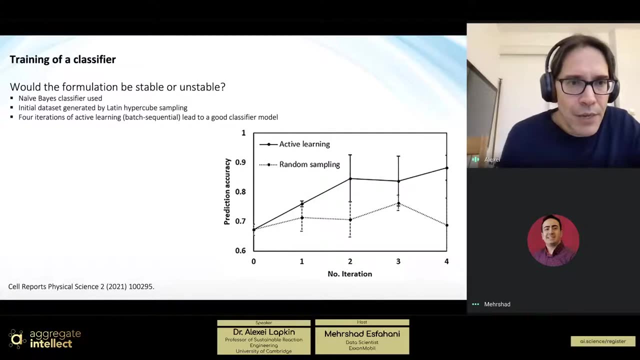 We haven't automated that yet, It's been done. And then we put it in the second robot, which is a measurement robot. It has some sensors and the viscosity measurements are done in a different system just outside. So first we trained a naive Bayes classifier. 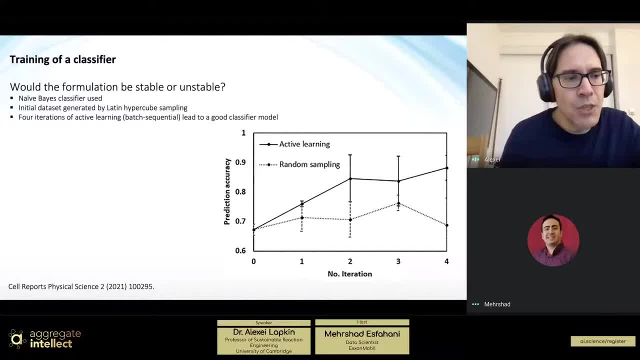 to predict whether the composition chosen by the algorithm is going to be stable or not stable. We've proven that the naive Bayes classifier is probably the best for this task And it certainly works better than the random sampling Then after that, after the classifier was done. 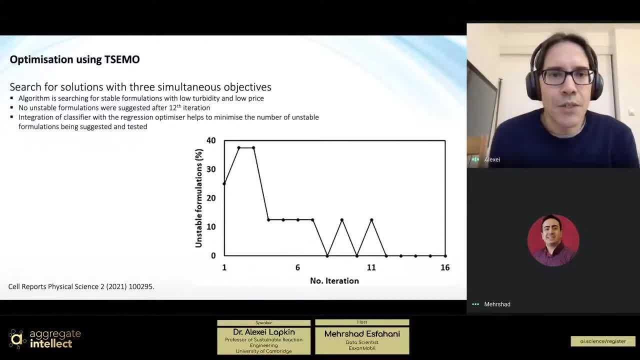 then we started regression And regression. within 12 iterations it no longer suggests any unstable formulations. So it still passes sub through the classifier. It still samples the space where you can have unstable formulations, but it's now looking for three targets: low turbidity. 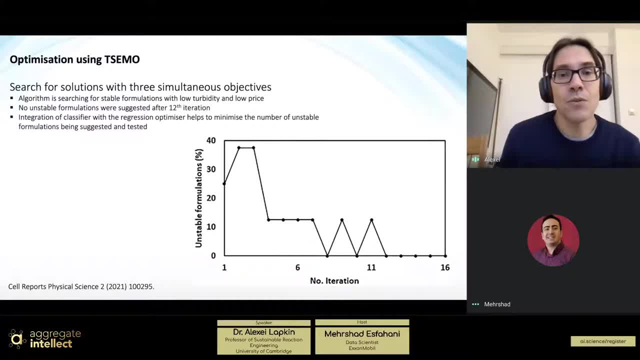 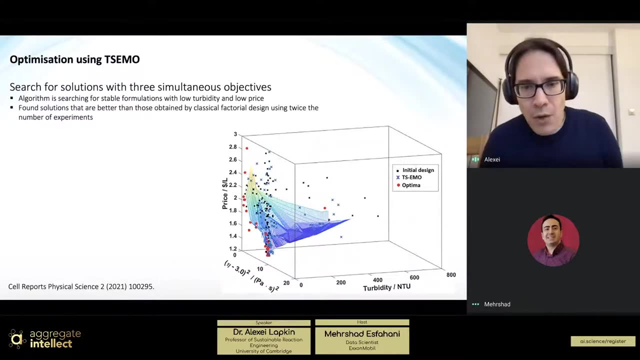 stable formulations and low price, And so low turbidity is also low because it corresponds in this case. So the regression algorithm helps in getting to formulations which are stable. And then if we look at how the entire optimization space looks like, 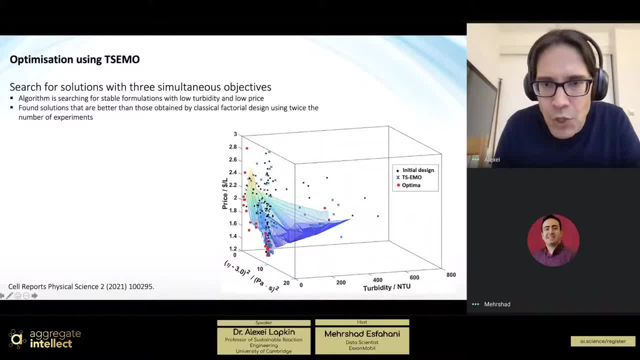 this is a comparison of the data points collected by the train algorithm, which is the blue crosses, the experimental optimal solutions. where we think is where the optimal solutions are these red dots and the initial design and the black squares. So you see, the initial design is all over the place. 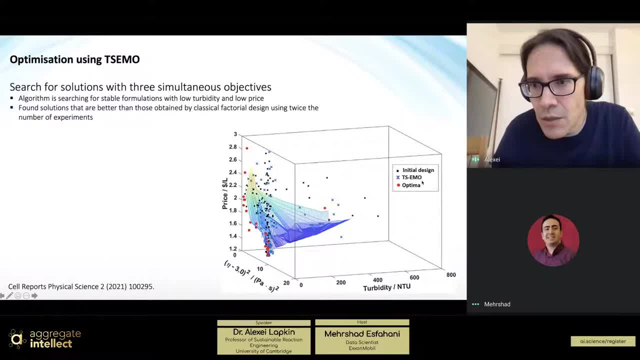 Again it's Latin hypercube. And then the optimal are the experiments where we're really sure that those are the good experimental data points. And then the TSE. more is the trained optimal solutions of the Pareto. In this case it's a rather complex Pareto surface. 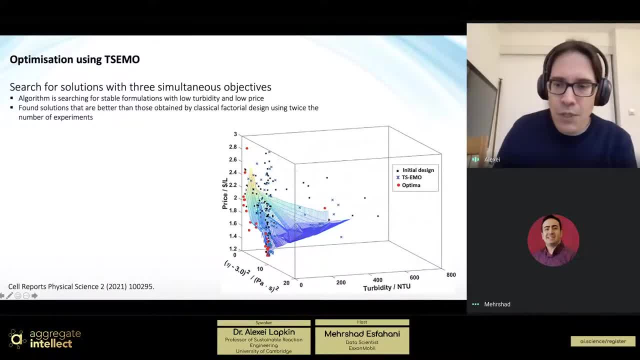 It's highly nonlinear space. But what was interesting in this study? we managed to find a number of formulations in half the experiments, a number of formulations which are better, lower viscosity and lower price compared to what the experimentalists could find just using purely factorial. 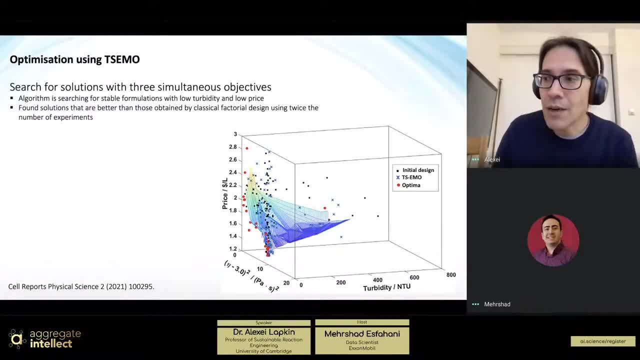 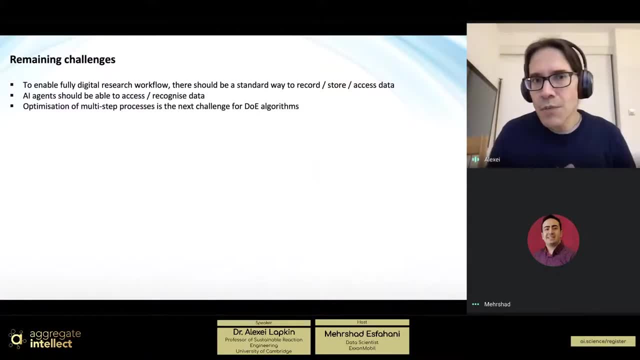 classical factorial design without any machine learning, in half of the time, in half the number of experiments. So this is everything I wanted to show. What remains for us to do, and where we put in most of our effort today, is to try to fully digitize the workflow for laboratories. 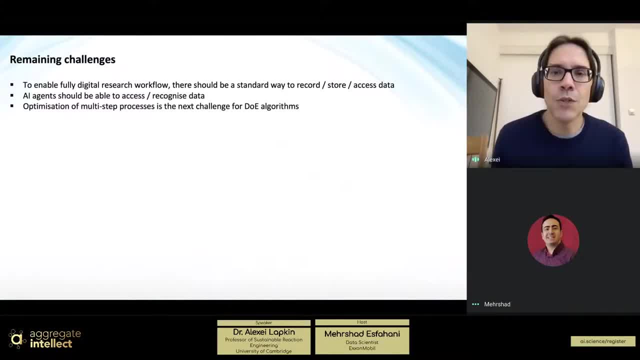 And this includes standardization of the way we record, store and access data. We then want to have a space for AI agents to play effectively. Our machine learning algorithms we treat as agents, And so we need to have the environment in which the agents could recognize. 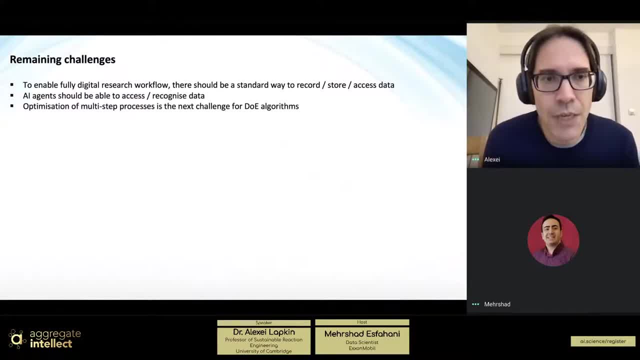 where the data are, what the data are and how to work with this data, And then on the specific chemistry challenges. the next challenge is the multi-step processes, where it's not a single step but two, three, four, ten steps in the process. 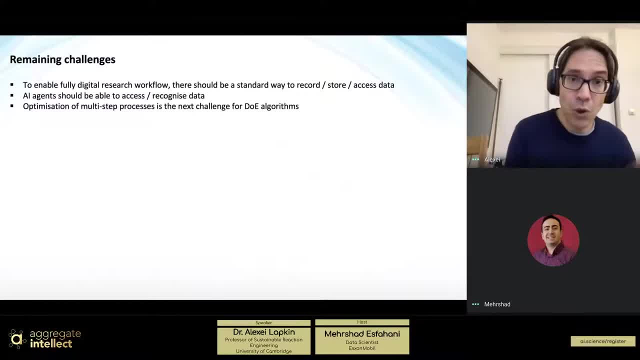 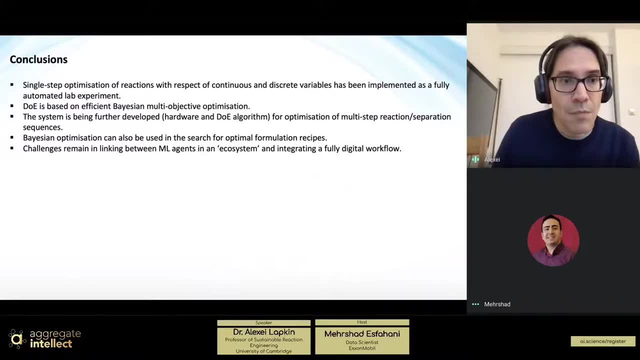 which need to be optimized for global optimum rather than local optimum. This is the real challenge for the DOE algorithms. So I've shown you that the single step optimizations are now, I would say, pretty much routine. The automation of lab experiments can be done. 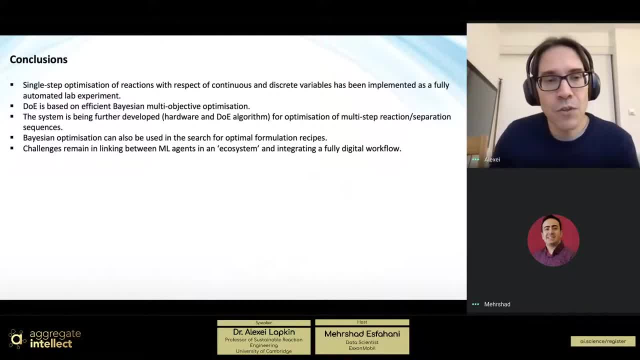 fairly straightforwardly. It's not very expensive to do. We work with multi-objective Bayesian optimizations. They seem to be quite effective. The system we are now further developing for multi-step reaction separation sequences. We've shown that same Bayesian optimization can also be used in finding optimal formulation recipes. 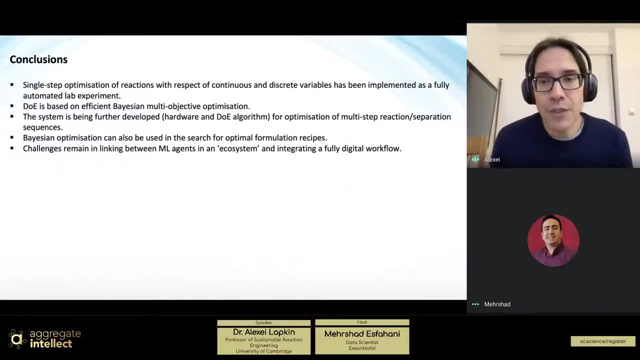 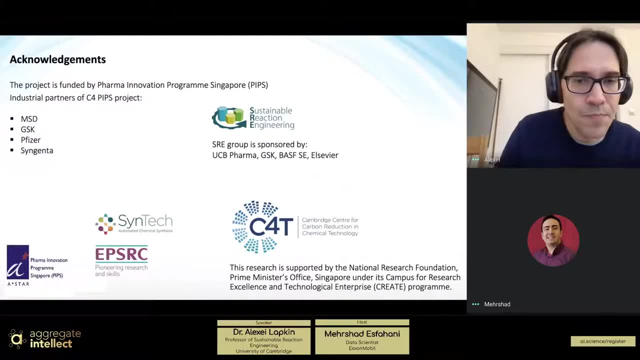 And then the challenge is to create this ecosystem of agents and data to have a fully integrated digital workflow. So I'll leave you with the acknowledgments of my industrial partners, the funders- public funders in UK and in Singapore- and also the acknowledgment of the contribution of students. 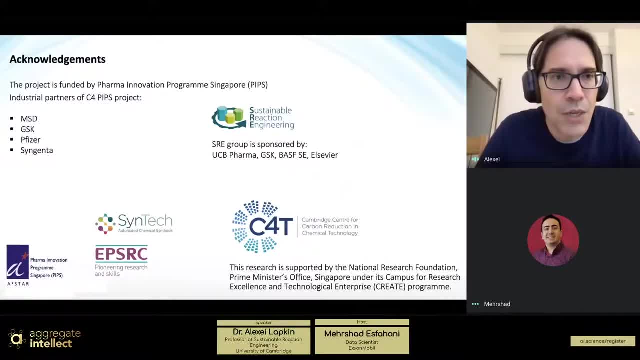 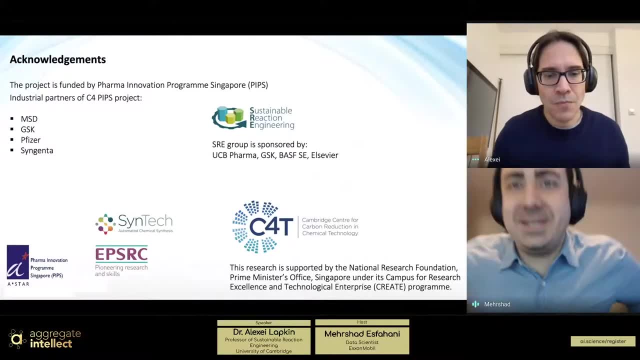 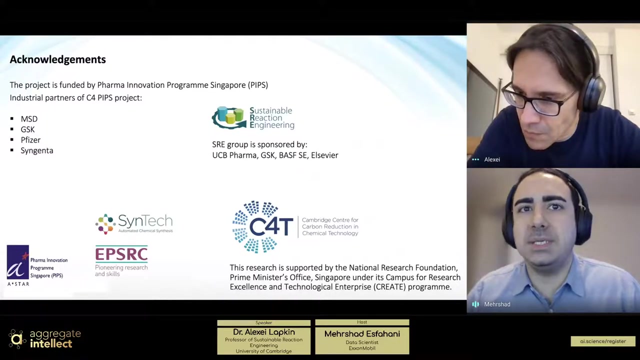 who are involved with the Syntec doctoral training center. I'll stop here, Sure, Thanks a lot. I really enjoyed it and it was very impressive. And just a few questions about the work that you have done. It appears to me that you used constraint nonlinear optimization. 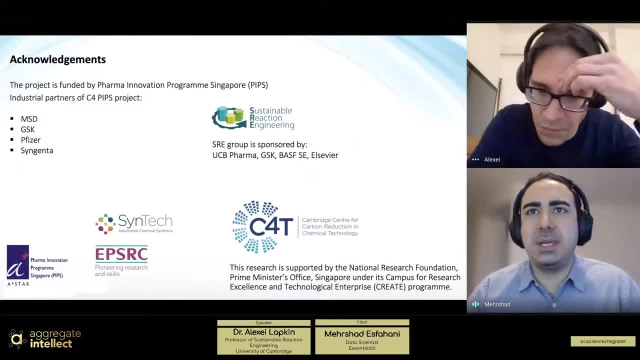 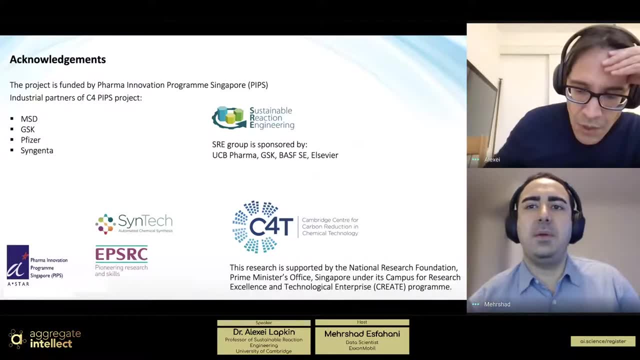 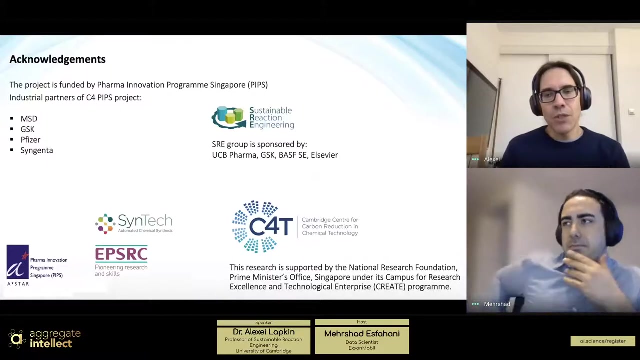 So would you mind explaining a little bit more the algorithm that you use for optimization? So we use an algorithm which is called TS-SIMO. We published it a few years ago. It's based on using a surrogate function, So we train Gaussian processes. 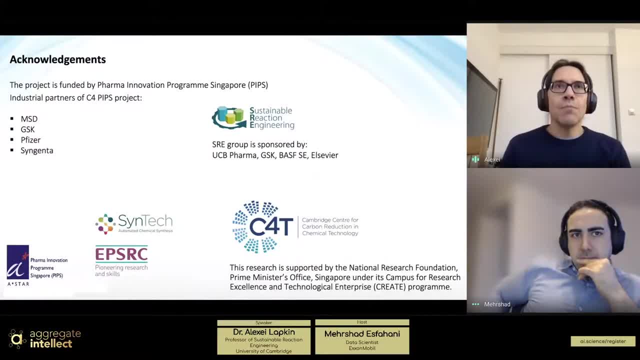 Then you need to sample from Gaussian processes So that you effectively create a sample to create predictions, so that you have the Bayesian approach. But then you also need to make sure that you do not have an excessive sampling so that you don't run too many experiments. 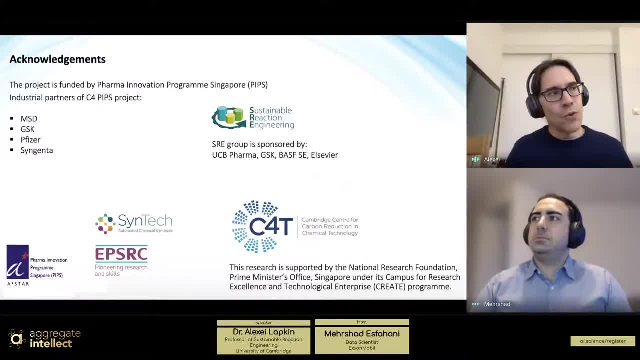 So you need to balance looking for an optimum and getting the right statistical function, So exploration versus exploitation. Then you can set up a certain acquisition function. There are a variety of acquisition functions which could be done. We used entropy in the first one. 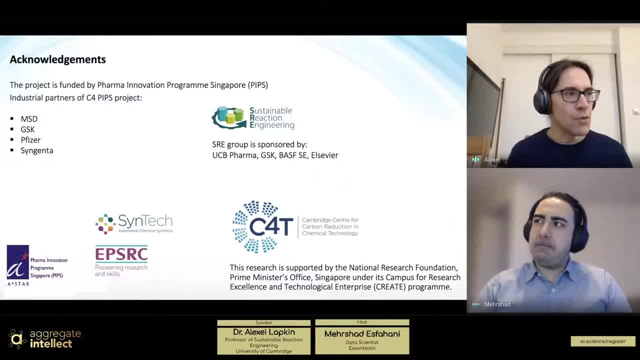 Then we use different functions later on. It almost doesn't matter which one. It's basically computational efficiency which gives you the choice of the acquisition function, And then you need to also choose how you sample. In the first algorithm we used, we basically had a grid search. 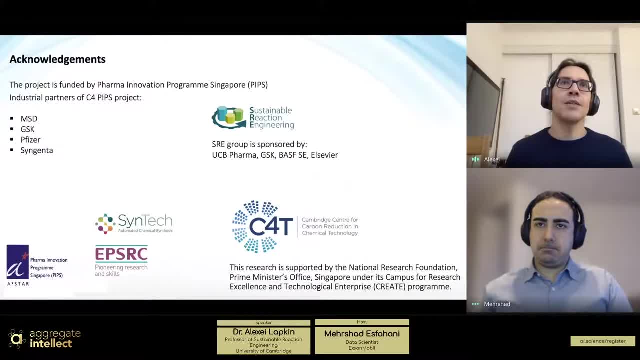 We said, okay, we're going to sample some points in the grid, which is okay, But you don't always need to do that. It's sometimes excessive, So you're doing excessive work. So in Tia Simo, the sampling is done. 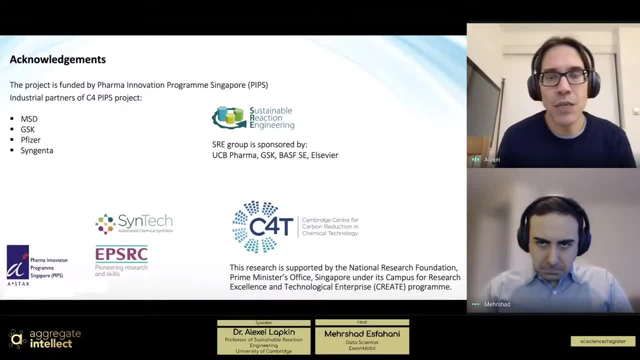 It's so-called Thompson sampling. So it's a spectral sampling technique which allows us to more efficiently sample from the GPs to get the overall model. So that's basically the way how this works. It's a non-parametric stochastic optimization And I saw in your slides. 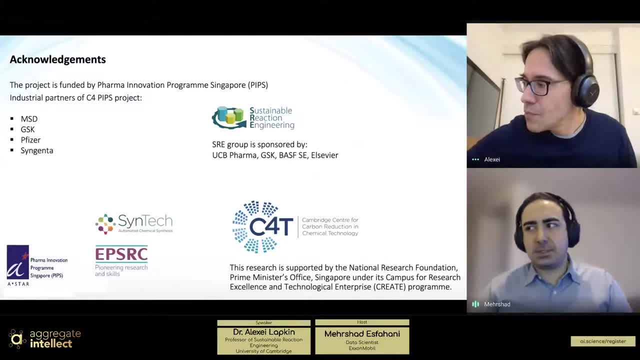 that reinforcement learning is part of the model, or at least is going to be part of the model. So is it based on this optimization or it's going to be used for this, to finding the probably global minimum, or is for some other part of the system? 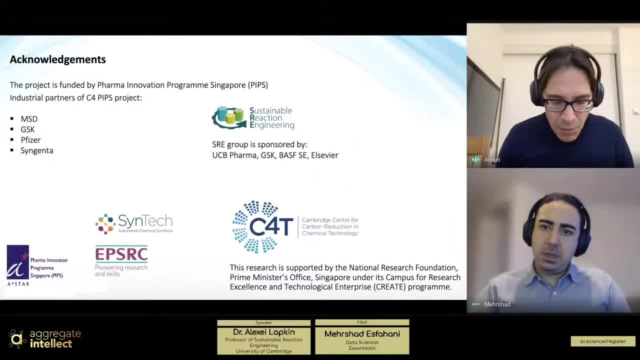 So reinforcement learning we already implemented as a tool to search for optimal policies to design superstructures in process development. So the paper have come out about a couple of months ago Now. it's a lot of people are interested in reinforcement learning also as an optimization technique. 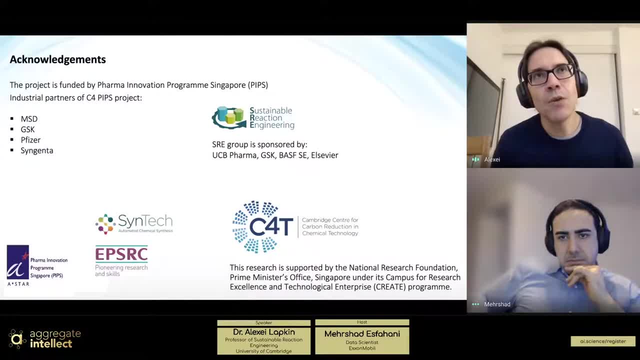 And so we will include the RL module into this benchmarking, just because some people want to use it. It's not the most, it's probably the least efficient one, But because people are interested in RL, we are working to include that into the summit package. 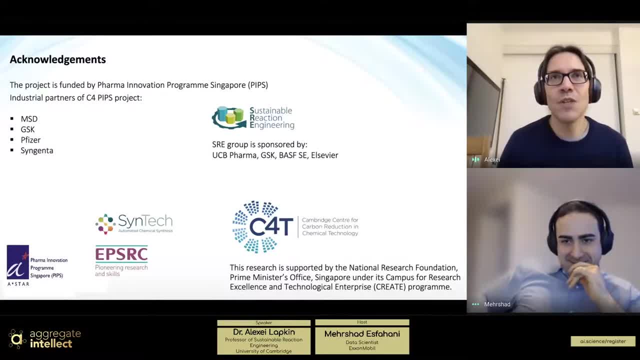 So it will be there. It's not there yet. It's almost finished. We just need to debug it and then it will be released. Wow, that's fantastic, And I saw that I'm guessing that you're using kind of a. 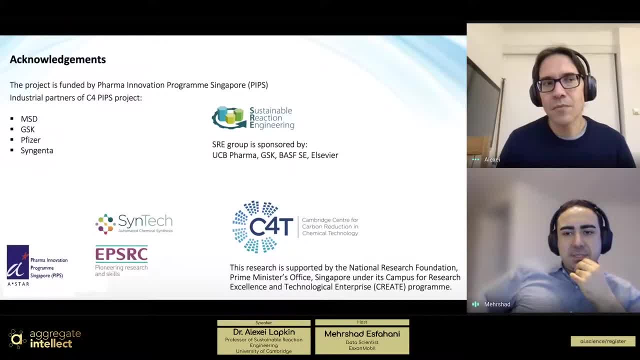 like binary classification to decide whether it's stable or not. So can you elaborate what criteria you're specifically using to decide whether it's stable or not? Is it just physical properties like temperature and pressure of this one, or there are some other? It's visual. 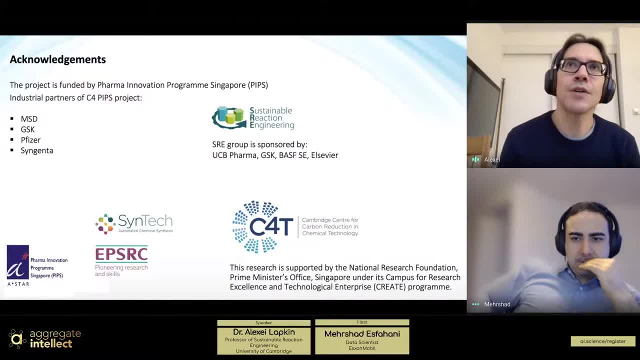 This is how it's done in industry. Formulations are characterized by the stability over time and it's basically your observation of the change of turbidity over time. So the unstable formulation will basically layer out And if you have an expensive experiment, you have cameras which take images. 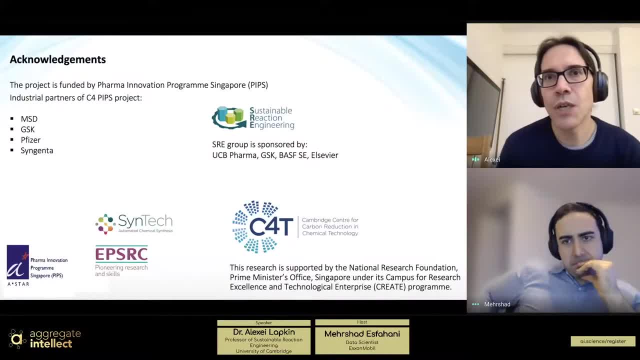 with different exposures and different lighting. We take one image, So our measurements are not very accurate, but they still give us an indication. So we have an image with image analysis and we have a turbidity sensor, So we take these two measurements together. 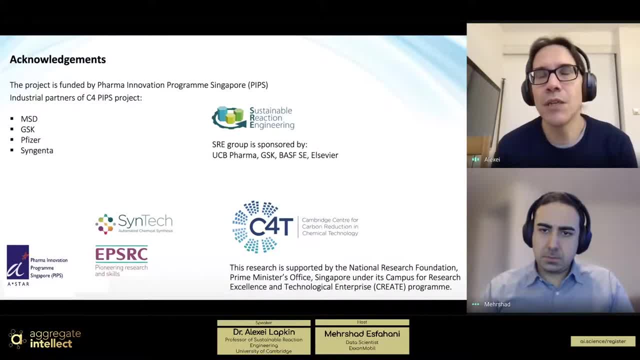 Whereas in commercial setups for analysis of stability, they measure turbidity and they measure multiple images which they combine together into a single indicator later on. Interesting And finally, for the software that you are using, like you showed us the graphical interface for someone who is not familiar. 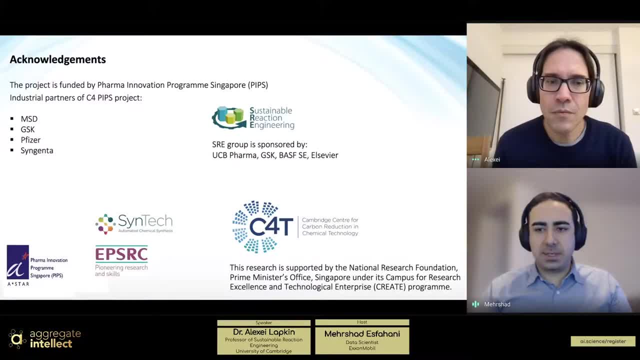 with machine learning. is it commercialized, If people want to use it or at least work with it? how is the process? The paper with this work is now out. It's open access. The MATLAB version of this algorithm and the interface is published on the GitHub.